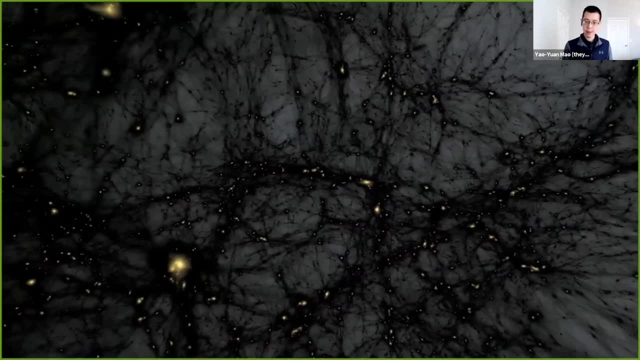 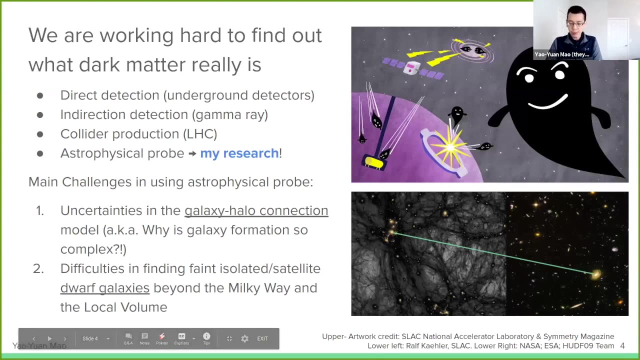 distribution in our universe. so so, um, what is dark matter? we still don't quite know what document is, and i mean in the past, i guess decade or even two decades. um, we have been working very hard trying to find out exactly what it is, and so there are many particle experiments. uh, they are searching for dark matter and in this very 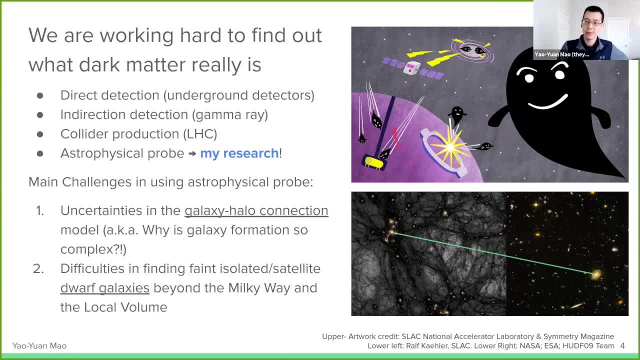 cute cartoon. they actually uh, show you three distinct methods that people are trying to find documented, including direct action, where we put a director underground so that only documented particle are more likely to pass to hit a director, to produce a signal. in direct action, where we are hoping to produce by annihilation of documented particles, and also, uh, through collider, this one. 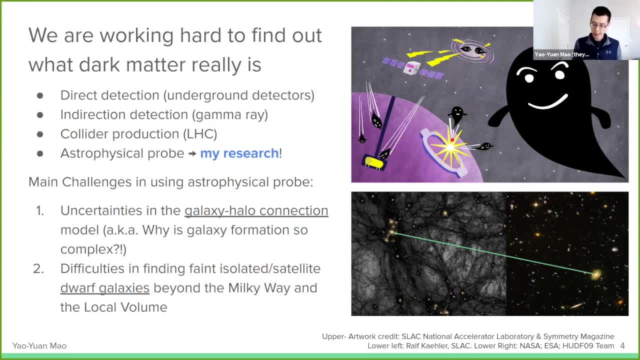 at the large hydrogen collider, we are colliding protons and hoping to turn energy into, uh, documented particles, and so these different particle experiments are ways that we search for, i guess, the signal of document, but we haven't found any through these methods so far. on the other hand, we have been 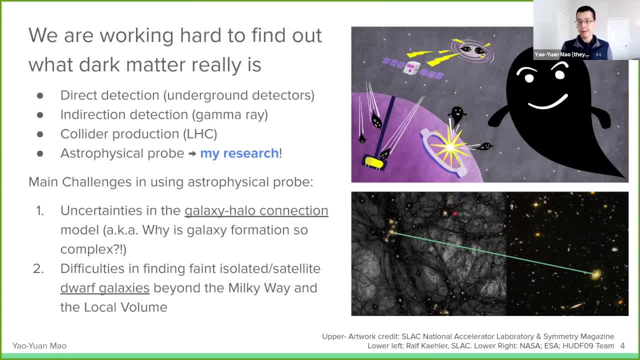 using galaxies and other astronomical observation to interpolate, I guess, provide evidence to the existence of the documenter, And so the question here is that can we take one step further to not only provide evidence but actually put constraints on the particle nature or non-particle nature of documenter? 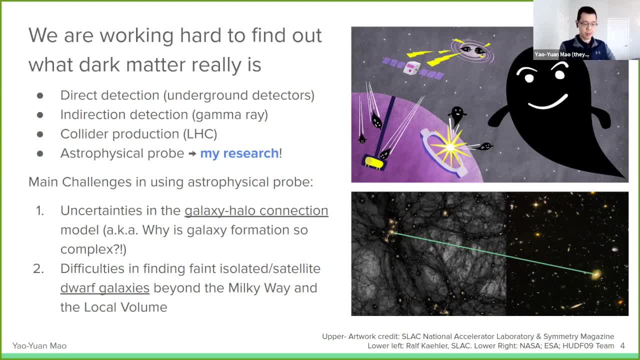 through observation of galaxies and other astronomical pools, And so my particular research lies in using galaxies. There are many other astrophysical probes that we can use to study a documenter, But for the use of galaxy, the main challenge basically lies in, I would say, two particular things. 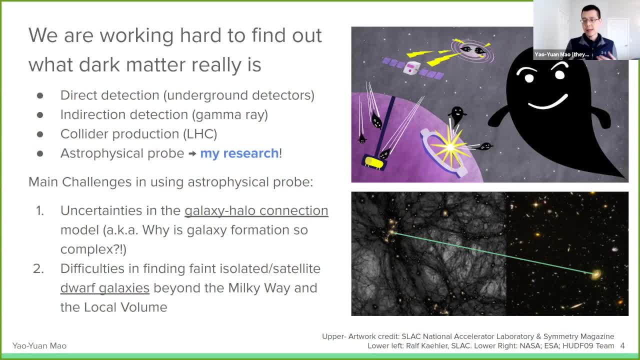 One is the uncertainty in a galaxy-halo connection. So, as I mentioned, in this very simple picture of galaxy formation, the galaxy forms within documenter halos, But there is a lot more physics involved in the formation of a galaxy, And so understanding how galaxy forms become critical. 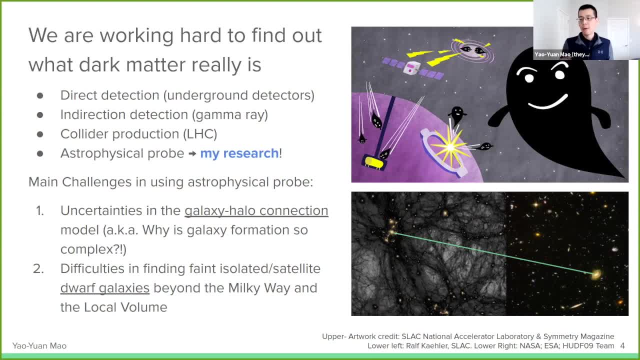 because that is one of the biggest systematic uncertainty when you try to use galaxy statistics to infer the documenter structure. The other thing is just: it's difficult to find very faint galaxies, And in my next slide I will show you why faint galaxies are particularly interesting. 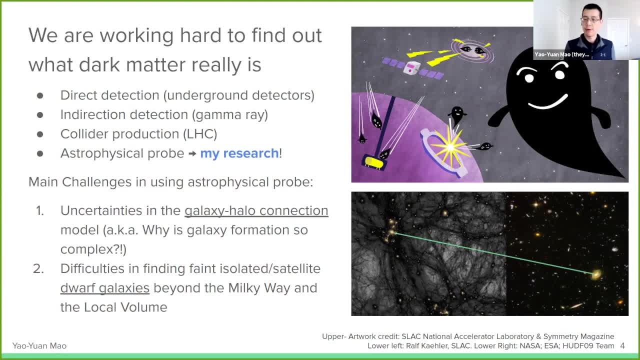 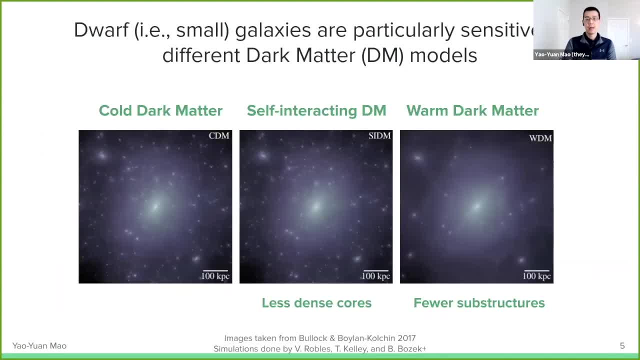 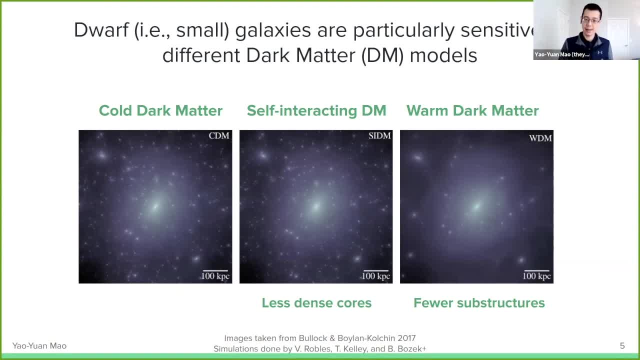 They are a slightly different concept. One is actual galaxies And the other is the duct substructures surrounding those galaxies, And so you are looking at the certain pictures of, again documenter assimilation with slightly. This one is a co-documenter, this one is a self-interacting documenter and this one on the right is one documenter. 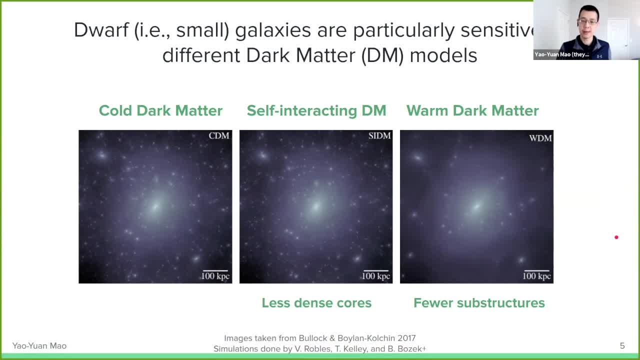 And so you can see they have slightly different imprints of the final substructure where we believe those would be places hosting those small dwarf galaxies. You can see very clearly: in the case of one documenter you have much fewer substructure compared to a co-documenter. 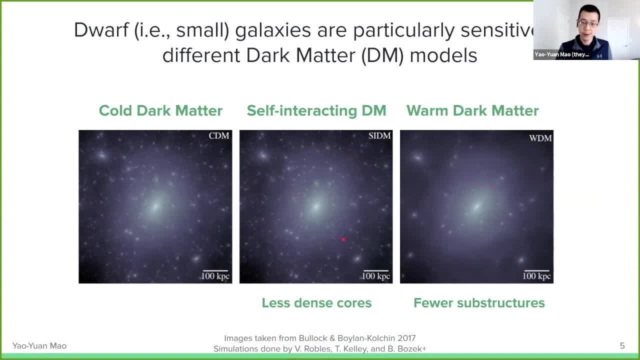 In the self-interacting documenter case it's slightly difficult to see this by eye, but if you stare at it long enough you will see. the density peak at both the center of the halo and also the peak of subhalos are slightly less peaky compared to a co-documenter. 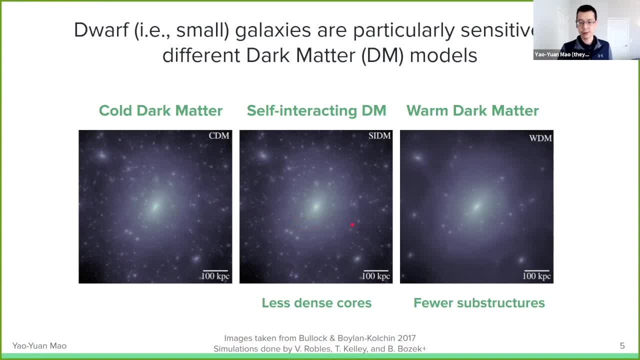 And that will also influence how a galaxy forms in those substructures. And so we believe, by understanding the population of dwarf galaxies in this kind of system, we will be able to put constraints on these different kinds of models. So what are these dwarf galaxies we are talking about? 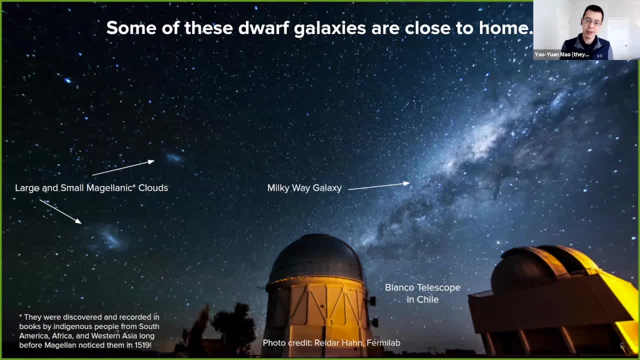 Some of these are actually. These are actually very close to home, And so here's a picture taken from the in Chile, near the Banco telescope. You can see our beautiful Milky Way galaxy on the sky, And you can also see the large and small marginality clouds. 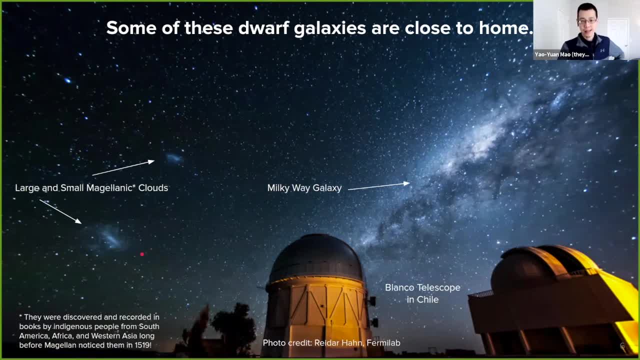 And so these are the two largest satellite galaxies that are orbiting our own Milky Way. They are living within, kind, of the Milky Way documenter halo, much larger than the Milky Way galaxy itself. It's about 10 to 15 times in size larger. 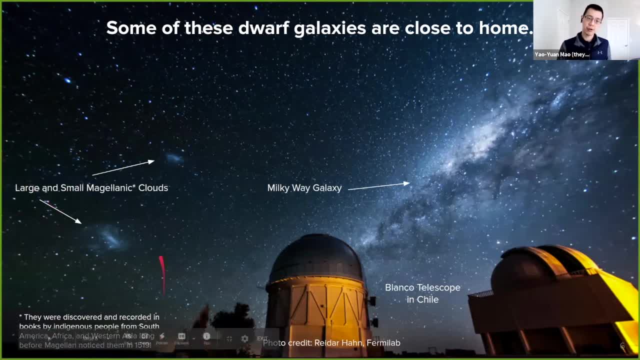 And so the smaller galaxy. these two galaxies are gravitational bound to the potential of the documenter halo and are orbiting the Milky Way, And so this is like two of those galaxies that we can even see by eye in very clear sky. 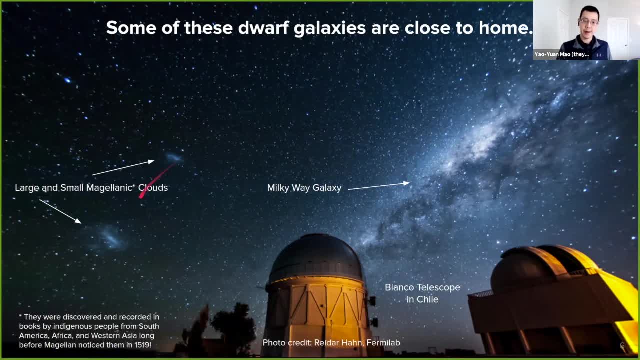 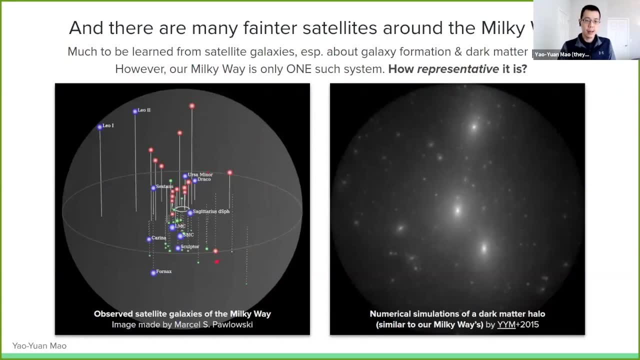 And there are many more in the Milky Way, much fainter than these two, that are orbiting the Milky Way. So here is another picture of the same thing, but I mean in a, I guess, illustrative way, And so you can see LMC, SMC. 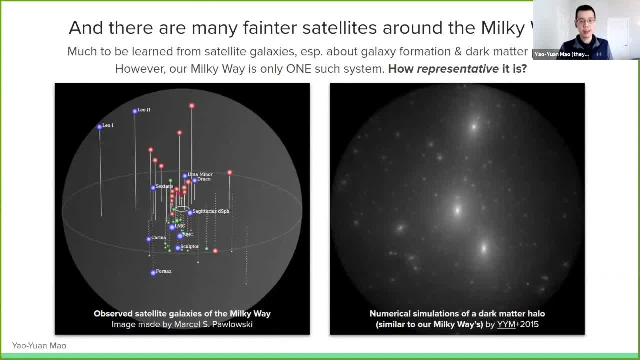 the large and small marginality clouds that I mentioned earlier and a lot many more satellites that we have discovered today orbiting the Milky Way. On the right hand side. I'm showing you a picture of a simulation that I ran earlier. This is the Milky Way sized documenter halo. 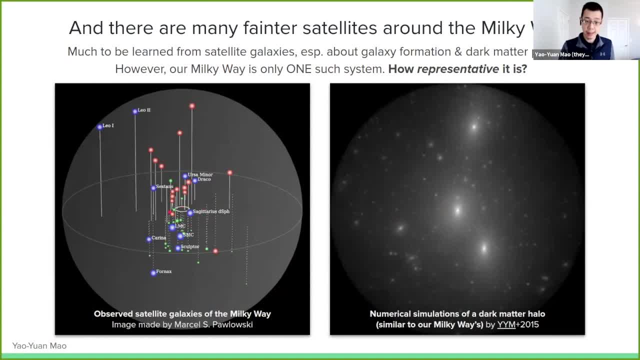 And, as I mentioned earlier, the Milky Way galaxy itself is much smaller compared to the size of the halo, And so these substructures, which we believe to host, like for satellite galaxies like LMC and SNC, are orbiting the Milky Way. 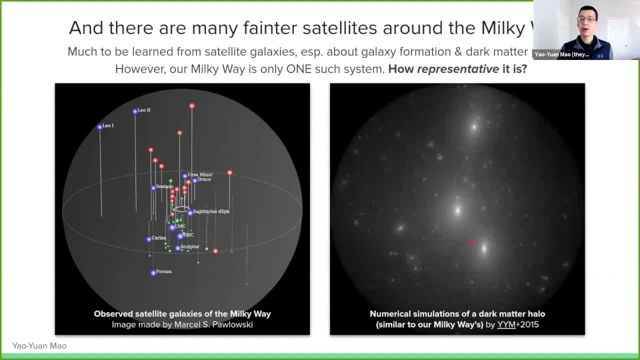 And so, by comparing what we observe and what we simulate, we are hoping to connect satellite galaxies that we observe with this substructure and then put a constraint on the documenter physics. But again, one of the difficulties is to really connect this particular realization of the satellite system with the simulation. 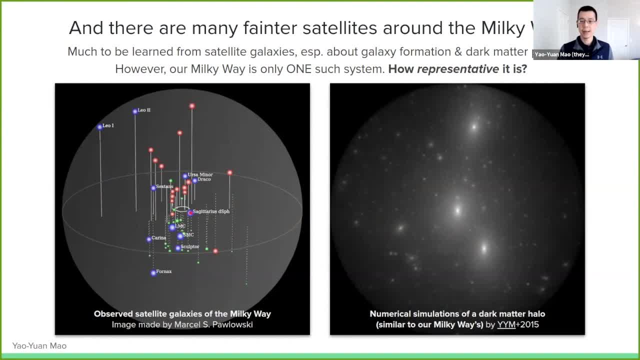 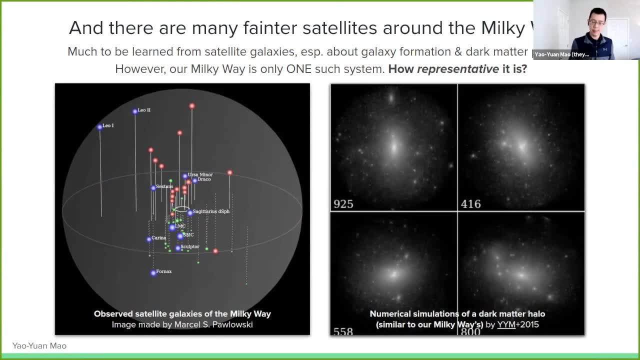 So how do we know the Milky Way is a representative, I guess galaxies in this halo mass range. In fact, in this simulation that I ran, we actually ran about 45 simulations. I'm picking just a random four to show you. 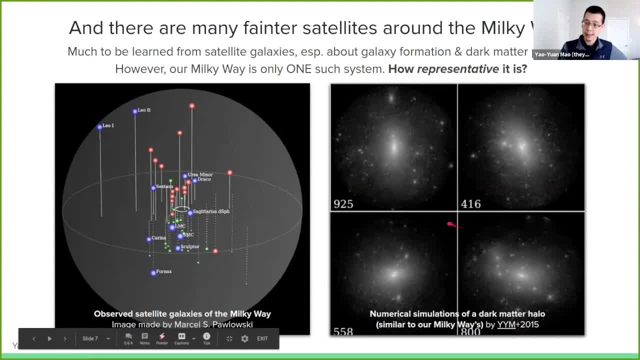 And you can see they have different. they actually have all similar halo mass, all these different simulations, But you can see they have very different halo shape. They actually have very different halo formation history and hence a different abundance of the substructures. 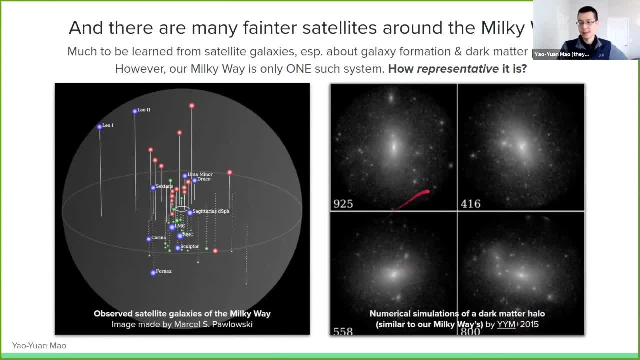 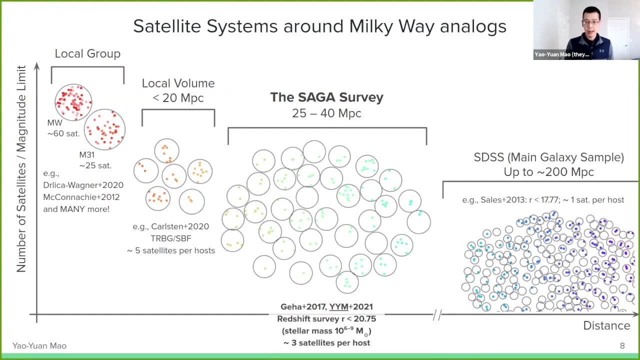 So, in order to figure out which one of those are more similar to our own Milky Way, we need that information in order to actually connect the satellites with substructures, And so, to that end, I have been co-piloting the SAGA survey. 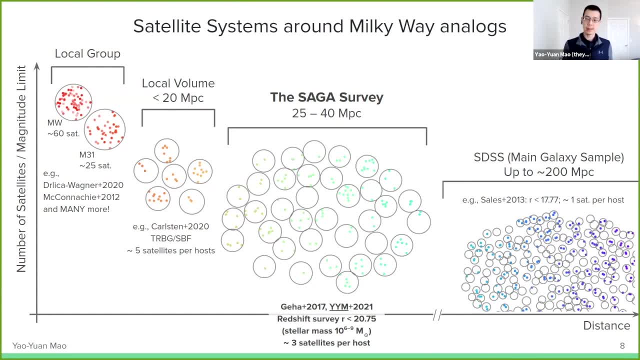 And the SAGA survey is to hoping to study satellite systems, like putting Milky Way in a cosmology contest, So having more satellite systems to study. And so just to say why this is it's difficult and put SAGA survey in contest with different other survey observations. 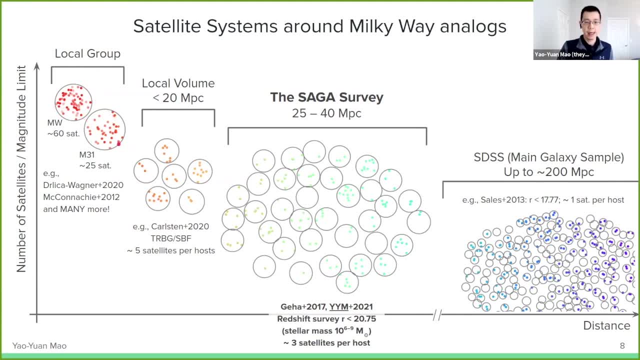 So in the local group we have the Milky Way, which we live in, and the M31, the dramatic galaxy that is our neighbor. They are really close to us And so we can detect to a much fainter limit As a result. 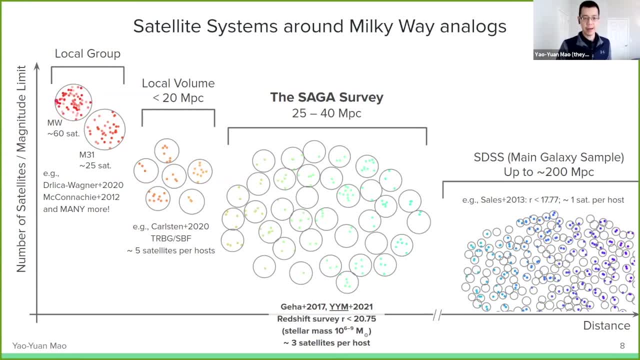 we can see a lot more satellites in those systems, Like in the Milky Way, I think right now we have about 60 satellites we have discovered in the Milky Way and about 25 in the M31. Once you move out to the local 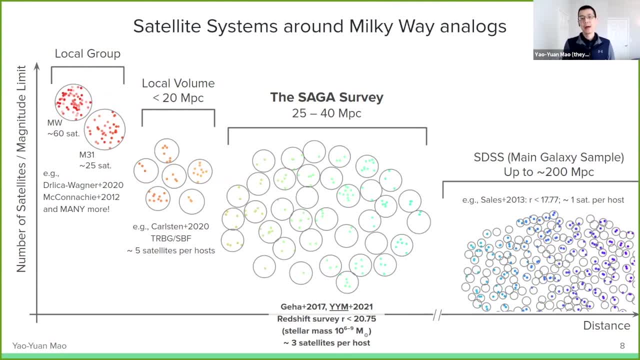 move outside of the local group and went into local volume, it becomes a lot more difficult to find the satellite galaxy just because they are much fainter and you need to measure the distance of those satellite galaxies, And so right now I think there are about six to 10.. 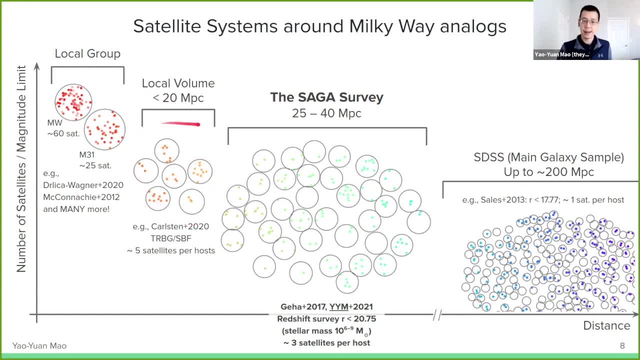 The number is still increasing rapidly of satellite systems that have been surveyed within the local volume. If you go a lot further and go to SDSS, the Stone Digital Class Sky Survey, and look at the main galaxy sample, you also find a lot of satellite systems there. 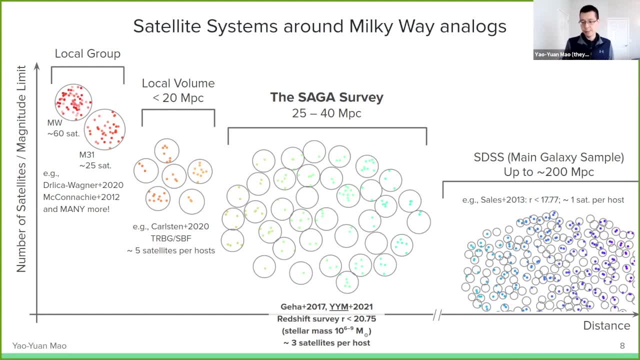 But again, this is a much further away, And so you can only detect usually the brightest satellite in those systems, And so on average you can have only one zero to one satellites if you use a Sloan Digital Class Sky Survey, And so the Saga survey is trying to put something in between. 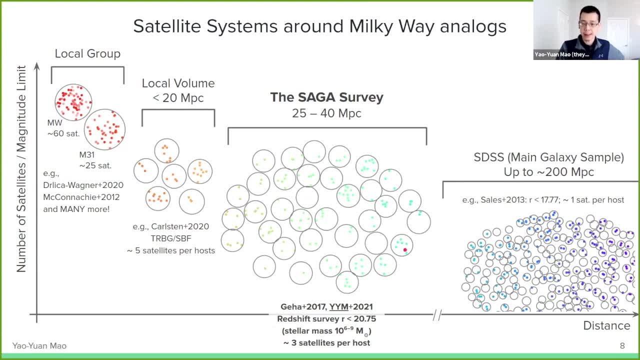 And so we are aiming for systems between 25 to 40 megaparsec, And our magnitude limit allows us to probe around three to four satellites per system, And so we are hoping to obtain 100 systems in the Saga satellite systems of Milky Way-like galaxies from the Saga survey. 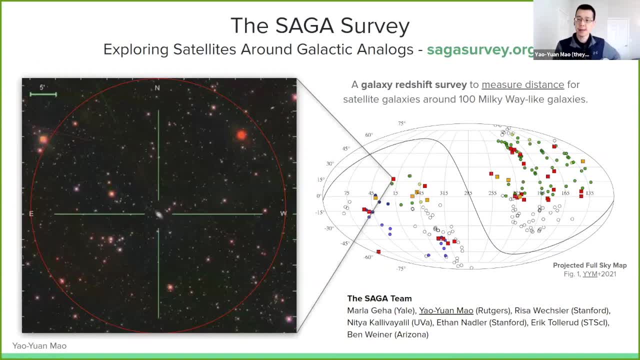 So here's just to show you the footprint of the Saga survey. As I say, we are trying to get about 100 Milky Way-like galaxies. We avoid the galactic plane just because there's high star population contamination for us, Not for others. 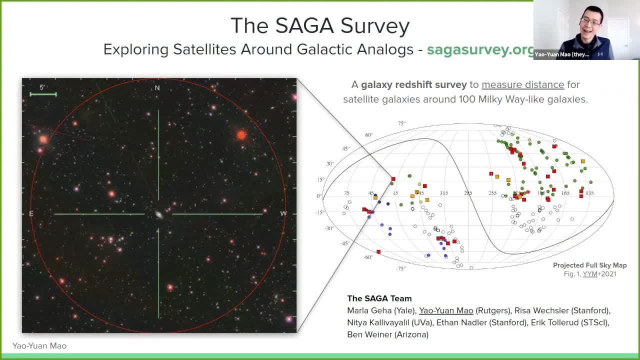 They are great objects to study as well And we, for each systems then we look into around 0.5 degree in radius, So this roughly corresponding to the viral radius of the corresponding dark matter halo And basically we are trying to find satellite galaxy in this field of view. 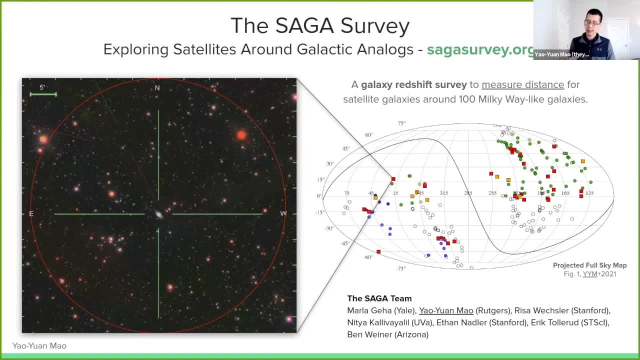 Because the distance is already further than 25 megaparsec. The way that we can measure distances by using spectroscopy- ratio, Tip, origin branch or surface brightness fluctuation- They are now applicable at this distance. We can probably use them for 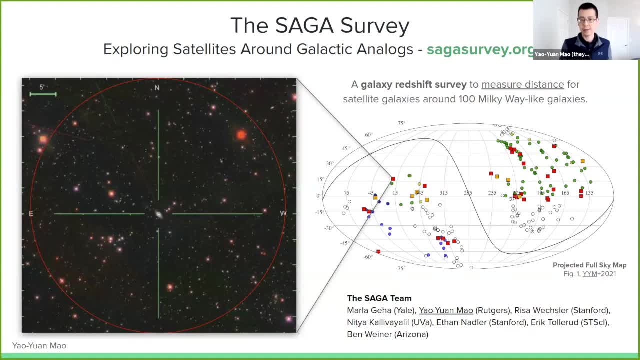 since they are within like five to 10 megaparsec, but not at 25 megaparsec or further. So in the end we measure the ratio for each individual galaxy, or almost all individual galaxies within the field of view. 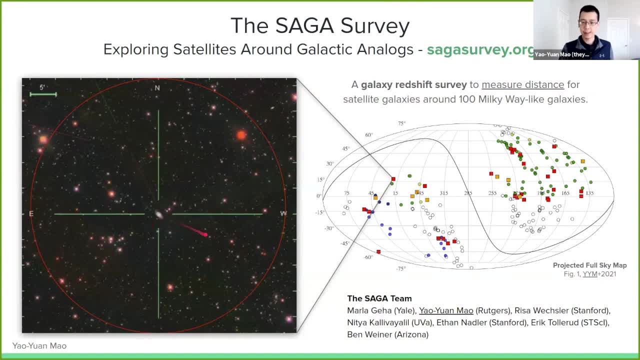 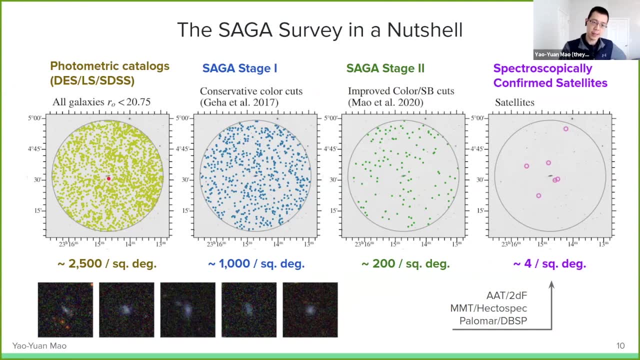 to tell if they are satellite galaxy of the host galaxy or not. So this is the Saga survey in a nutshell, right? So within the field of view, as I showed you earlier, down to our magnitude limit, there's about, I would say, 2,000 to 3,000 galaxies in the photometric color alone. 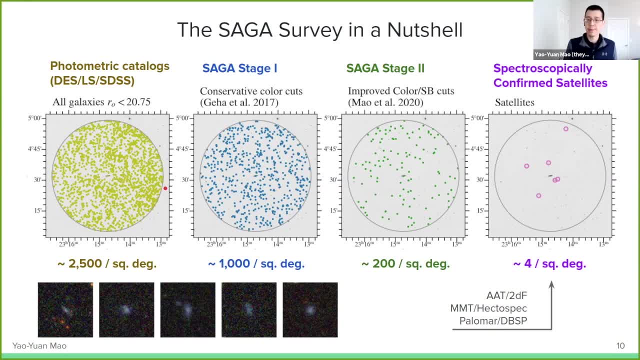 Most of this are just background galaxies. I mean, we know that because the background has much larger volume than since they are in the foreground, And so our job is to find which of those are actually satellite galaxy that are in the foreground right. 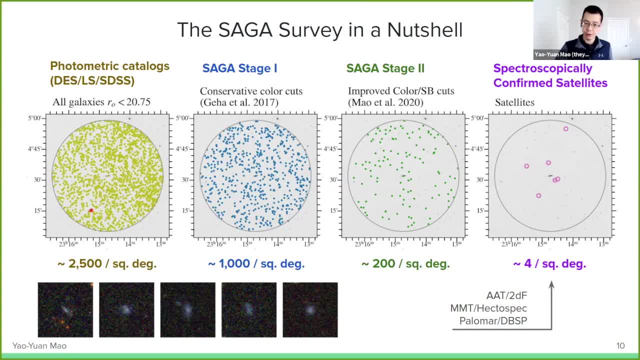 They are not background galaxy Because since in the background are redshift, they have much redder color. You can make a very safe color cut just to remove things that you know absolutely that redshift outside of the possible color range of full galaxies. 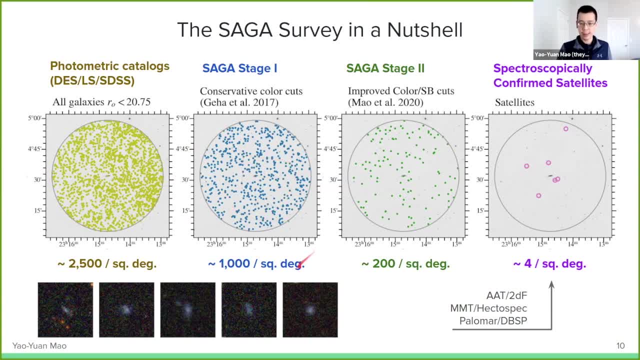 full dwarf galaxies And that will give you about still 1,000 per square degree left in the field of view. And so, in our first stage- Saga survey from 2013 to 2017, we took redshift for each individual object. you see at this conservative color cut. 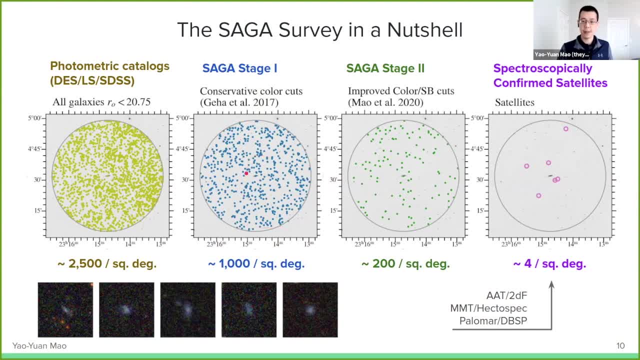 to obtain a very complete sample for the objects, And so from there we accumulate a lot of redshift data And from there we can actually do a much better training, And also partly thanks to deeper photometric data that later become available. 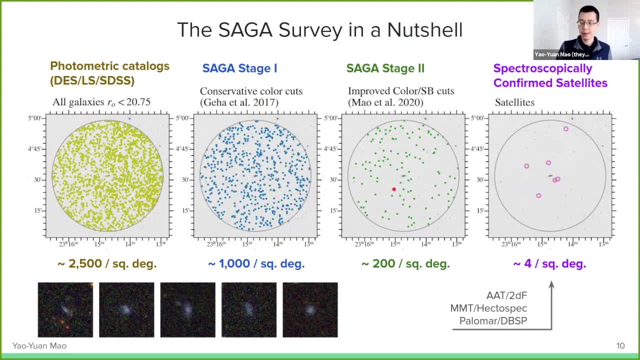 we then can actually improve our photometric cut, both using color and surface blindness, to further reduce the number of object candidates to about 200 per square degree, And so this make our- I guess- observation much more efficient. From here to here. 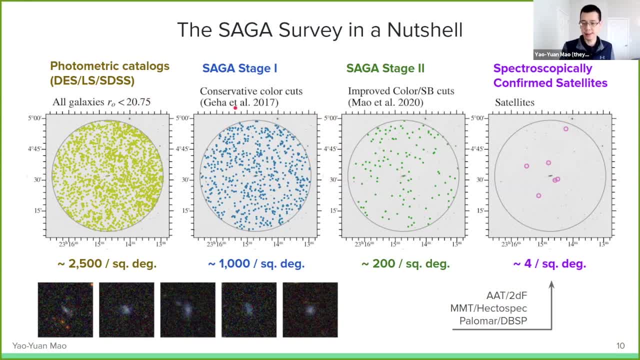 it takes us about like four years to get eight system to complete, And from here to here it took us about another three years to get, I guess, 25 system complete. So we are, like auto magnitude, increasing our observational speed with this improved photometric selection. 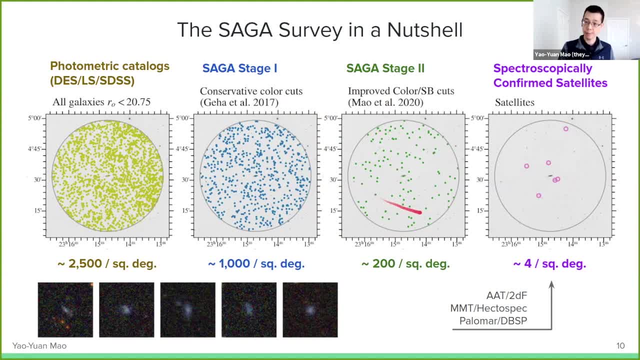 And in the end we still obtain ratio for each individual objects for this, because they are all possible candidates. So we obtain individual ratio for each of the objects and confirm the satellites. And this is just a set of images to show you why this is really difficult. 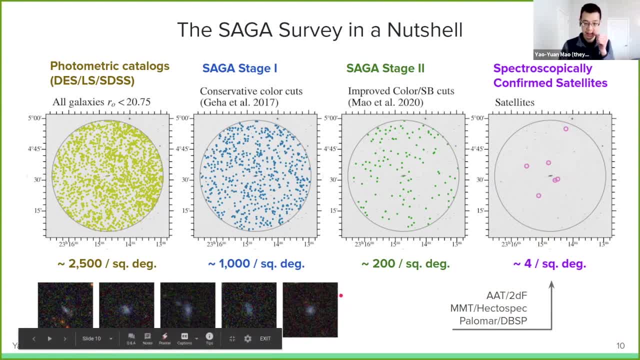 One of this is a satellite galaxy, a SAGAR satellite. The other four are background galaxies And you can see just from the photometric image itself. it's really difficult to tell which one is a satellite galaxy and which ones are not. 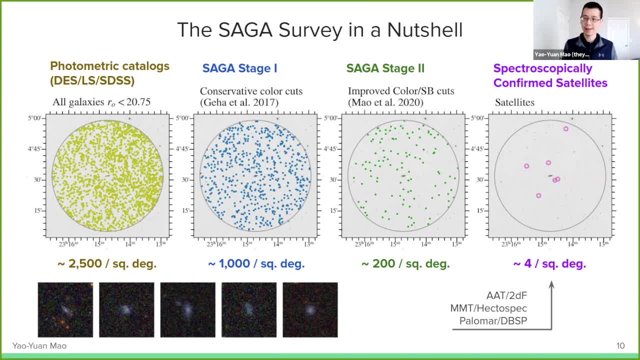 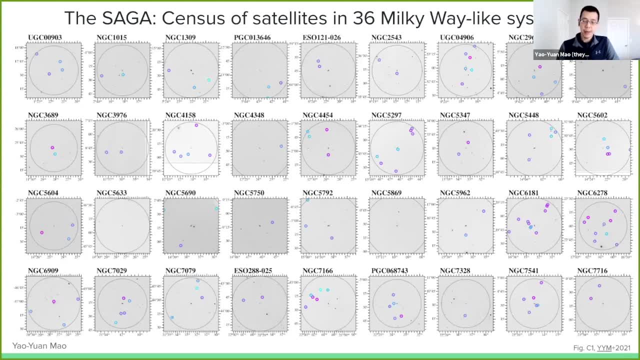 If you are interested, you can guess which one is a satellite galaxy. I can tell you the answer later. So last year we published our stage two result which we have: 36 Milky Way system we fully surveyed, And so you can see here this. 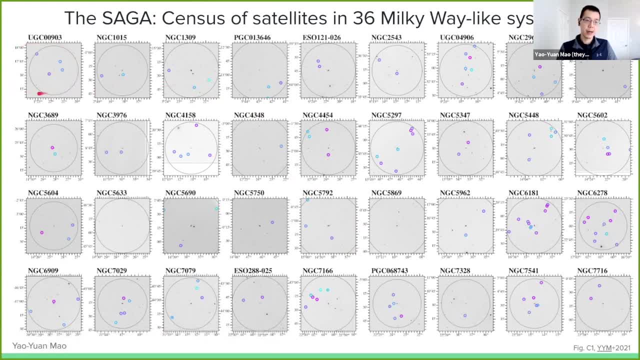 again field of view of the corresponding halo radius And all the colored circle are satellite galaxies we found. You can see that in some system we have very few or zero satellite galaxies. We found downtown magnitude limit. in some system we have like nine or 10.. 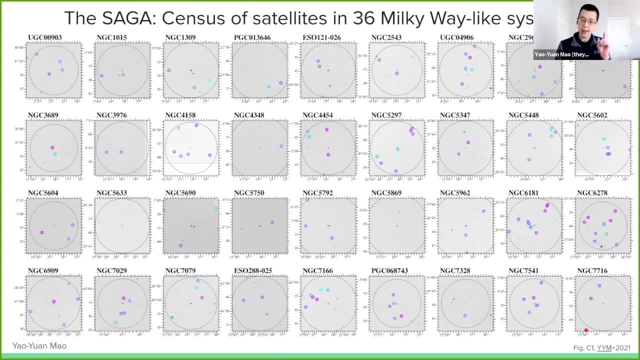 So this gives us a configuration space And the color is actually the line of the velocity. So it gives us some idea of the configuration and the velocity distribution of the satellite in the systems. Here is an image of the individual satellite we have discovered. 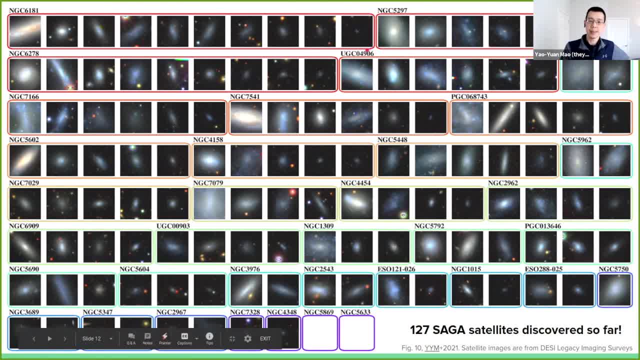 Each group is one system. So again, you can see systems with nine or 10 galaxies and systems with zero galaxies. You can see a wide range of different mobologies of the satellite galaxy. You have things as bright as, like the Magellan cults. 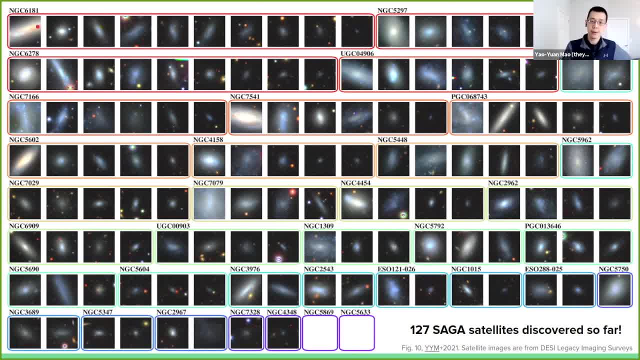 or even more structured than the Magellan cults, And you have this very tiny, irregular trove of galaxies, like little blob in the systems. I have a wide range of dynamics of this satellite systems. So there is a rich galaxy formation and galaxy evolution science we can actually study of these objects. 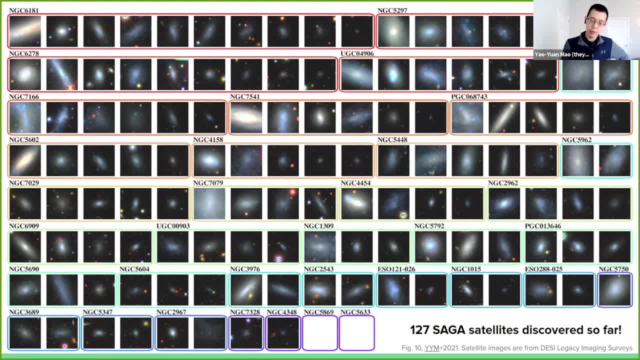 I will touch this only briefly, but I want to go back to my original talk about how do we use this to study the nature of dark measure. So you can see, for each group we can count the number of satellites, And actually the satellite here is ranked by their luminosity, from bright to faint. 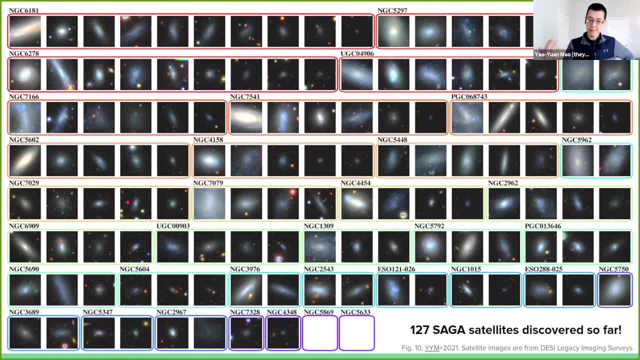 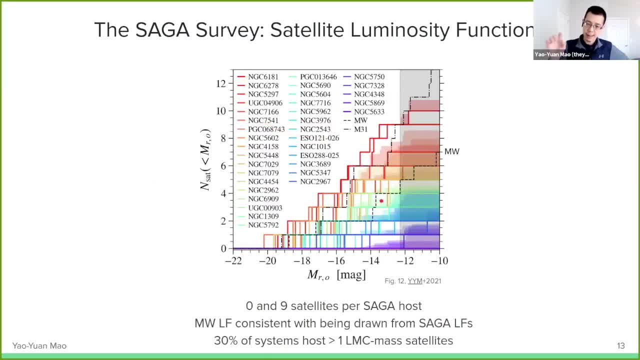 And so if I take the luminosities and plot the luminosity function like the number of satellites that function, luminosity, this is what we get Here. the color is the same set of color that you see earlier that are used to group each objects. 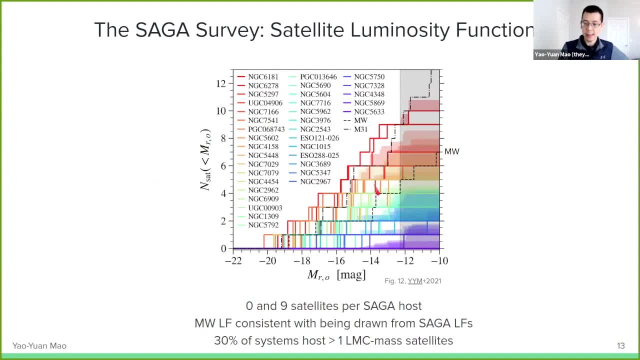 So you can see you have system with nine or 10 satellites. two systems have zero satellites. Again, this is observational program, So there's always some incompleteness, for example the ratio of value. And so all the incompleteness are modeled in our program with this shaded region that you see here. 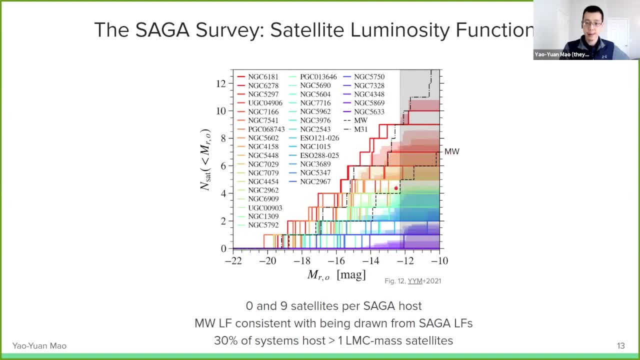 And so from here you can see the micro luminosity function, which is this line. It's pretty much, I guess, typical compared to the set of Saga luminosity function. There is actually an interesting thing, The fact that you see this. 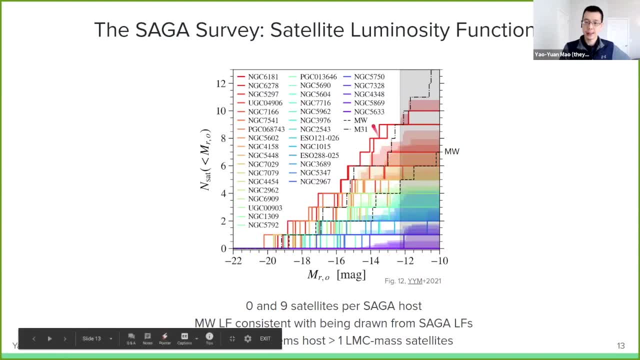 like a rainbow color is actually interesting. It actually means the set of luminosity function do not cross each other that often, So the system that have more satellites also tend to have more bright satellite, And this is actually expected in structure formation, if you only think about dark substructures. 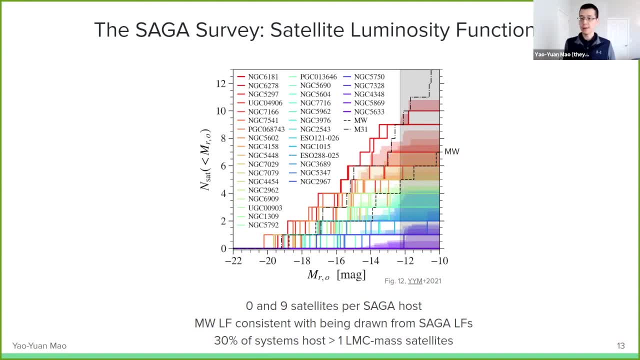 But the fact that when you look at the satellite distribution they also follow it actually means that the satellite actually follow the ranking of the halos quite closely. Like the stochasticity in galaxy formation function is not enough to totally erase the self-similarity in the sub-halo distribution. 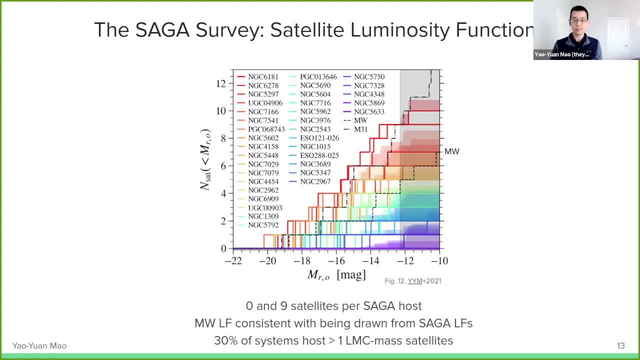 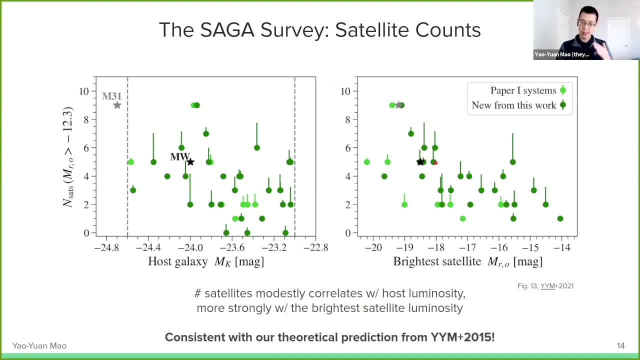 the sub-halo luminosity, the sub-halo mass function. So here's another way to see a similar thing. So this spread in the luminosity function. they are correlated with the host galaxy K-band luminosity. So this is the number of satellite as a function of the host galaxy K-band luminosity. 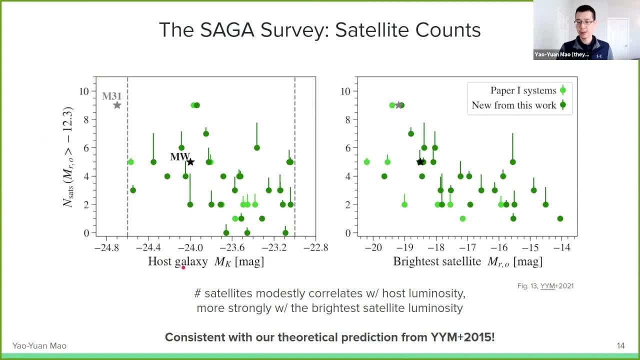 which is a tracer for stellar mass, And we also know that it's a correlation with the dark metal halo of the system. And so you can see there is a kind of a correlation there, kind of we expect, since they are brighter, are more massive. 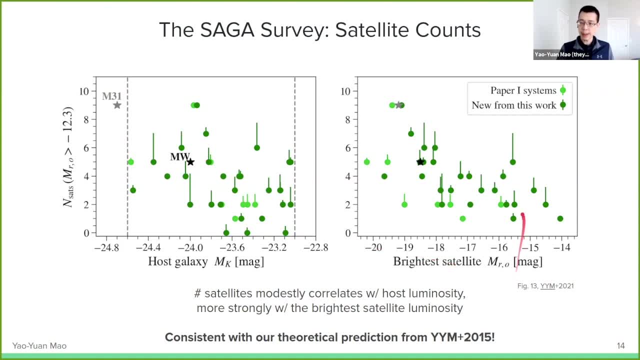 and hence they host more satellites. It might be interesting to know that the correlation is actually even stronger if you correlate with the brightest satellite, And this is related to what I say. This is what you actually respect in, uh, traditional structural information of 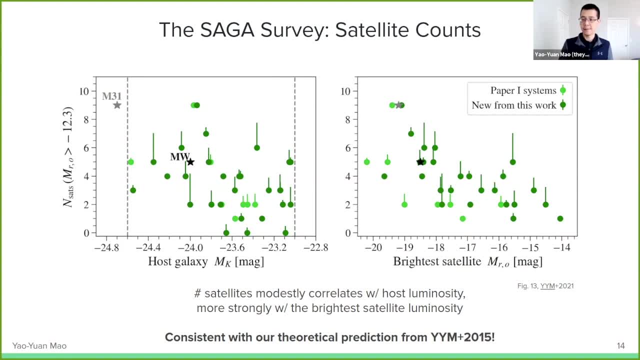 uh, dark metal universe where the brightest satellite kind of detect where the normalization of the sub-halo mass function is, And so the fact that we also see that in observation is really interesting and confront our theoretical prediction of that. the satellite follow quite closely with the sub-halo mass function. 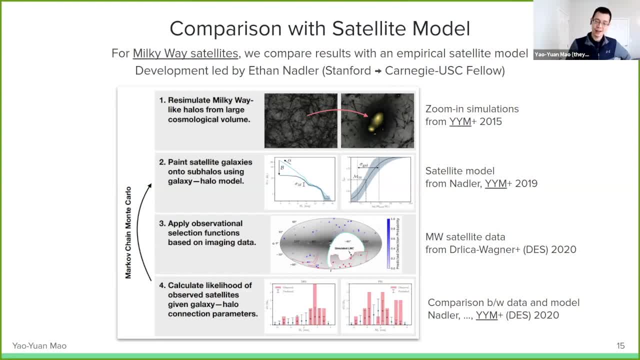 So keep moving on to how do we use that whole information? uh, to constrain dark metal. So I'm going to take a step back and just demonstrate how do we do this within the MQA, And so this is a series of work. 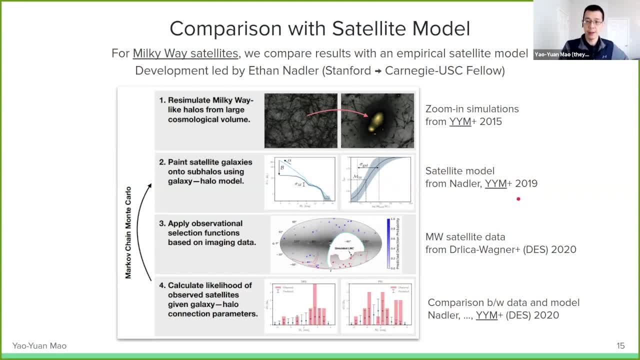 uh that by uh a student who I also co-advise at Stanford, Isa Neller. Uh, we use the satellite discovered by uh Sloan, uh all the classical satellite satellite discovered by Sloan Pan-STARRS. 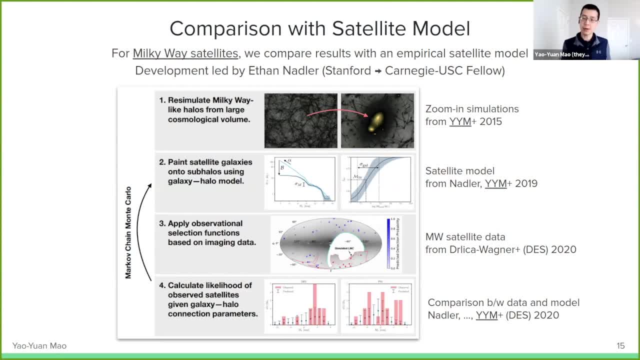 and Dark Energy Survey, DES, and then jointly model their distribution within the MQA. And so we start with the suite of simulation that I ran earlier, and then we apply a satellite model. So the satellite model is a connection of substructure to 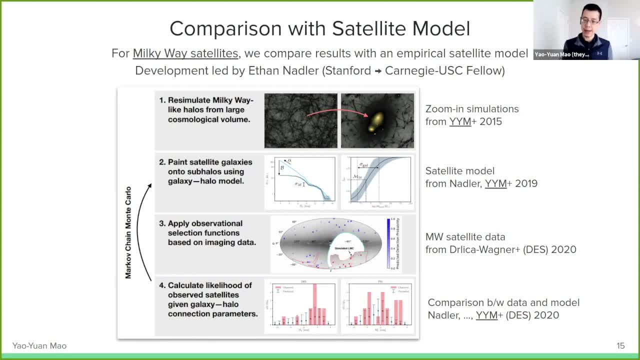 uh galaxy satellite galaxies mostly based on uh sub-halo bonus matching. So that is an empirical model connecting uh, dark metal halos and uh and galaxies, But we include a few uh recipes uh. 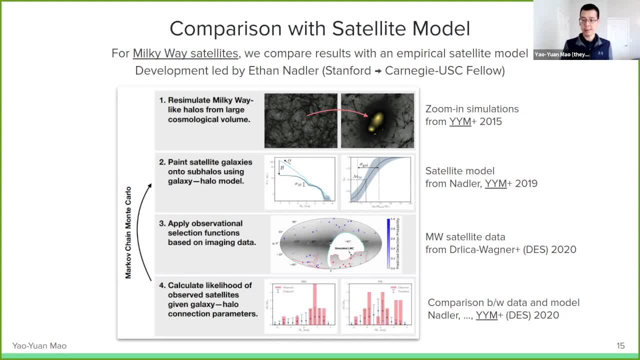 to take into account, for example, the disruption due to the central galaxy of the satellites, And so it's slightly more sophisticated than uh plant abundance matching technique. And then from there we applied them to the MQA satellite data and compared between the data and the model prediction. 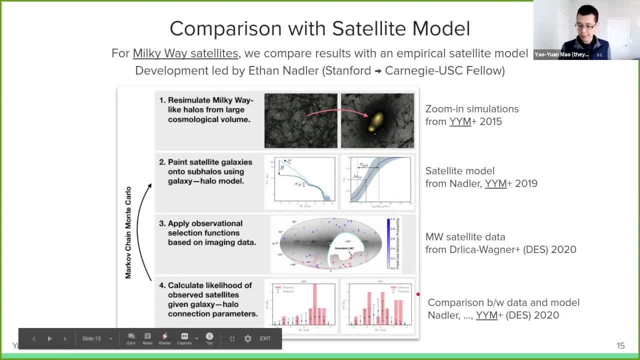 And so we run a multicolor, uh, multicolor, in order to get a full prior distribution. And so this, the dark metal part, hasn't come into here. right, This is just more, uh, kind of constraining the satellite model itself. 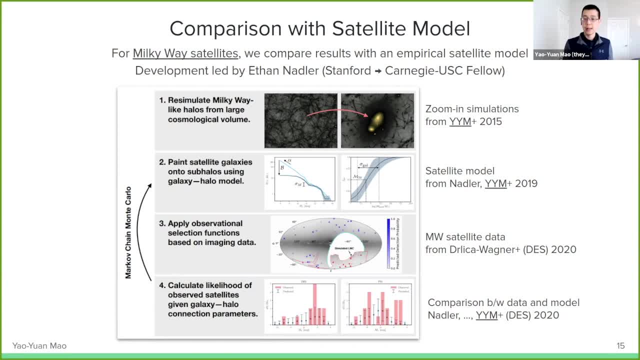 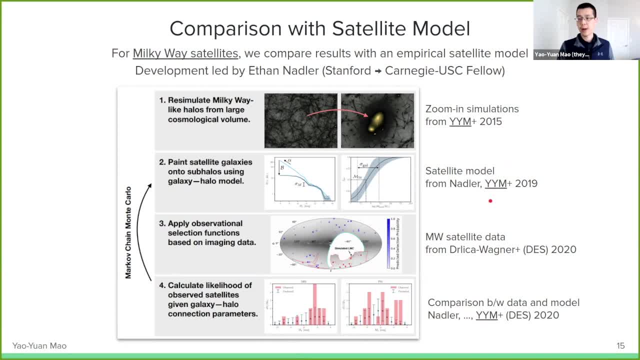 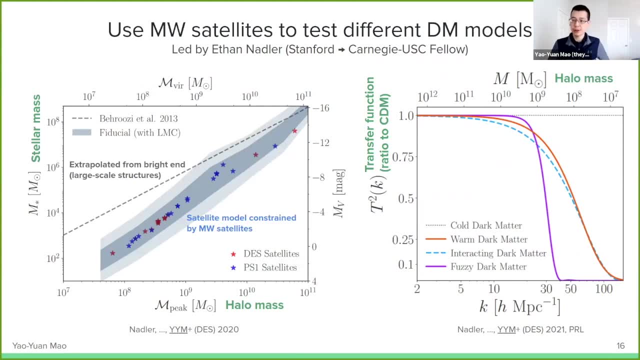 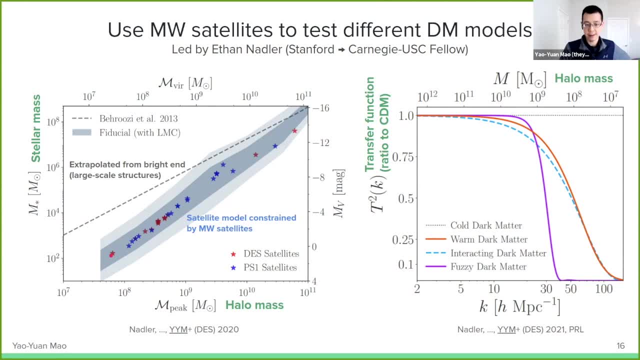 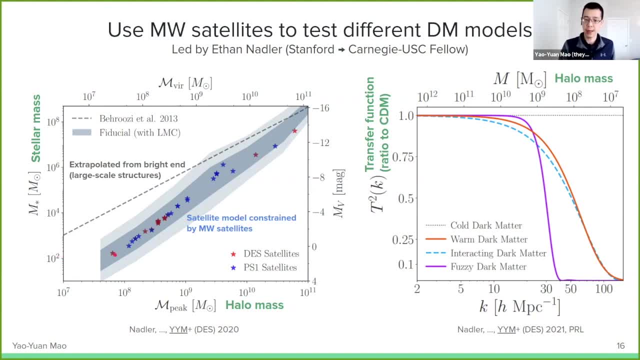 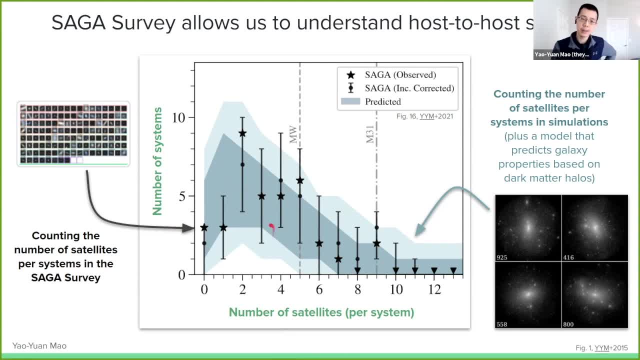 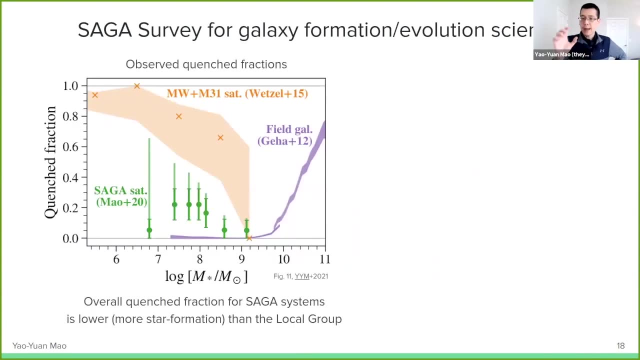 context of the saga observation, you can also see we still have quite big uncertainty due to the limited number of uh subsurface system. in saga we have 36. however, uh, we are on track to get more. so i would just say very rapidly that the saga survey, in addition to documented science, is also 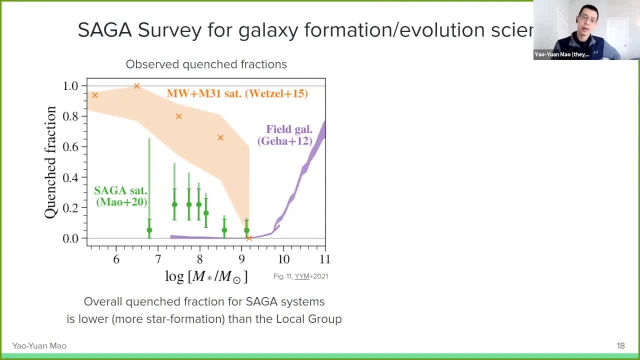 very interesting uh to study galaxy formation evolution, and so here you are looking at the quench fraction or the number of uh on uh now forming star gap satellites to the total number of satellites as a function of certain mass, and you can see the cycle points roughly here and they are kind of lower than the nuclear m31 satellites. 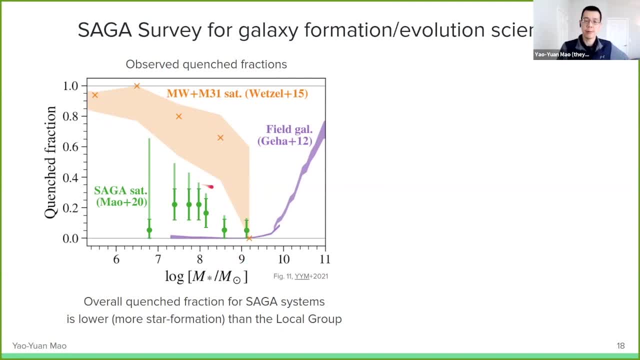 and so this has been. we have found this in our first stage result, but now we have a lot more data. uh, we still see the same trend persists, and so this is something that interesting, and we are eager to investigate what what this means to us, and we have been working with people running. 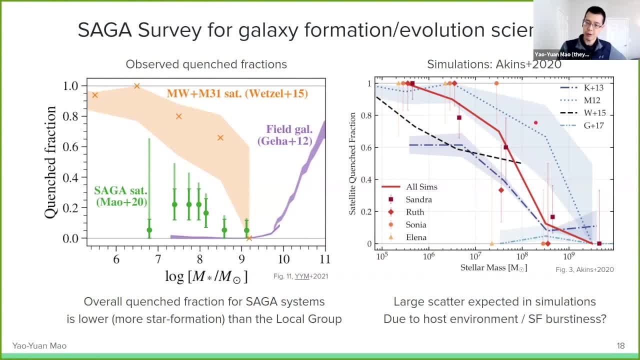 hydrodynamic simulations to compare our data with prediction from hydrodynamic simulation. this is one example for atkins from the embodied shock group of the hydro simulation. as you can see, the saga data kind of actually lie in between some of their simulated data. so this is one of their simulation goes from here to here. the other side goes from like here to here. so 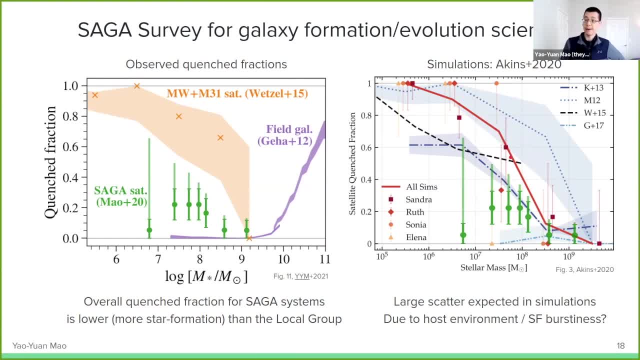 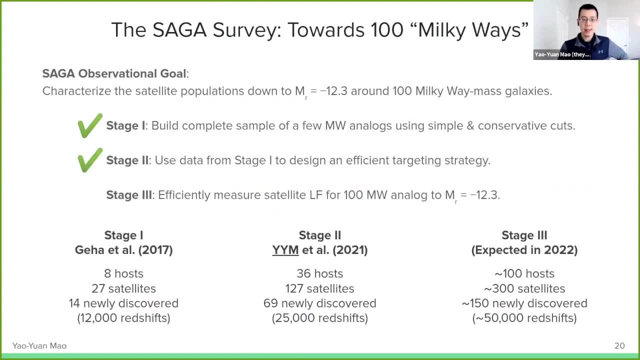 maybe the different hosts actually produce systems with very different uh crunch fraction in their setup population. i'm going to skip this slide, and so i mentioned that we have 36 hosts right now. actually, as right now as the time i'm speaking, we have uh 75 systems. 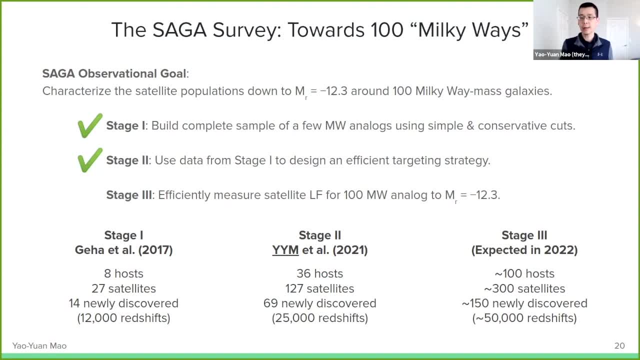 that we have completed our survey and we are uh expecting to complete the full survey to reach 100 hosts by the end of this year and publish our result uh- i mean they this year early uh. next year, and particularly uh, we will also discover about 50 k rush shifts uh that are newly collected by 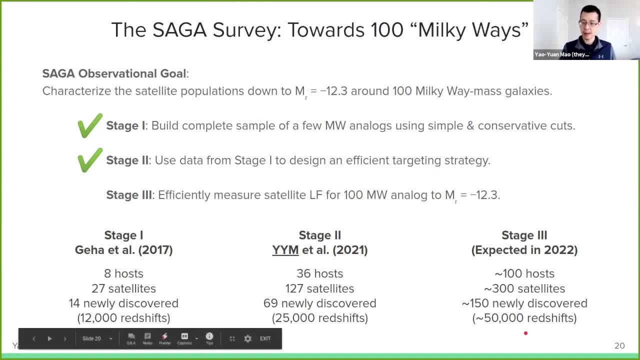 the saga king and this redshift uh will also have a lot of additional science that we can do with the data. currently we don't plan to uh expand the saga survey, so the saga survey will kind of come to a completion by the end of this year when we reach 100 hosts. 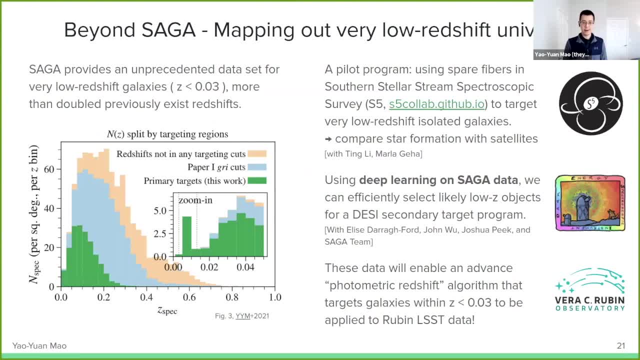 but it's good to think about what scope beyond the saga survey and in particular, as i mentioned, we have the tons of redshift that we collected in saga survey. they serve us practically uh training data for very low range of universe, because the saga survey is focusing on like zero, point one. 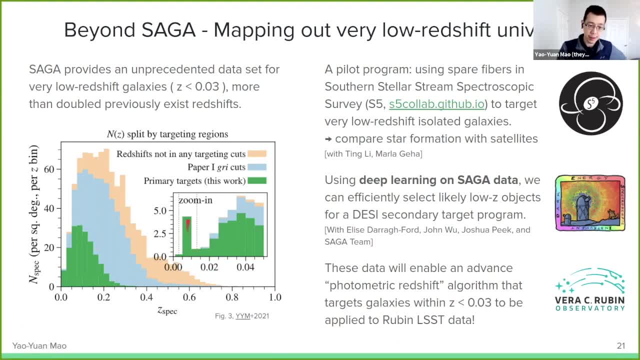 uh, in terms of ratio, right. so this is the ratio distribution and this is where the saga supply lies. so we have actually been quite successful in obtaining, like spare fibers in other programs to just do a very low ratio survey. so in particular we have been working with the southern study. 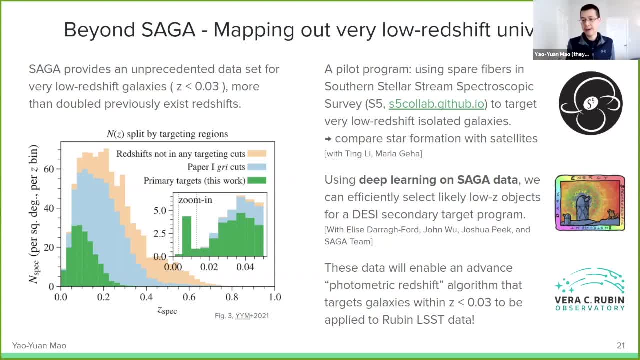 stream specialist copy survey, or s5. we just put in spare fibers using the saga photometric selection and trying to get, in this case, isolated, very low ratio and friend drove galaxies, and we will be able to compare the sub-formation history of those isolated galaxies and satellites. 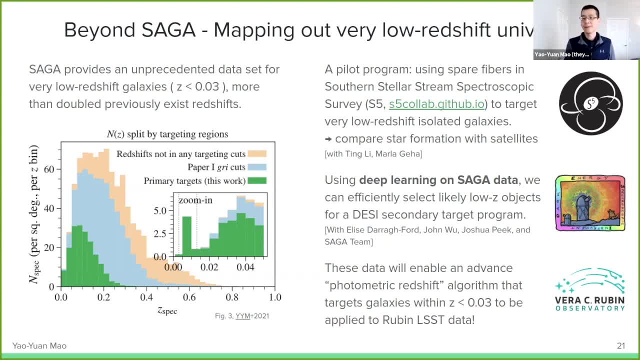 We have also been able to convince DESY to give us some of their secondary targets in the program. I think they are actually going to have a survey, like starting one of our programs this week And again, this will survey a large portion of the sky and we will get a lot of I mean. 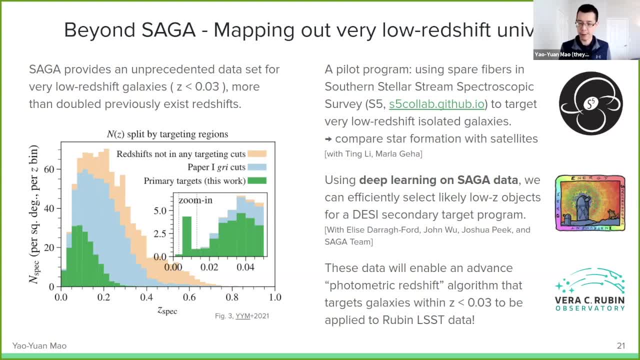 we are hoping to obtain a lot of very low ratio of galaxies. So by very low ratio I mean ratio of less than 0.03, and that map out the local universe down to like a standard mass of 10 to the 7-ish. And in the future I'm hoping to lead this program. 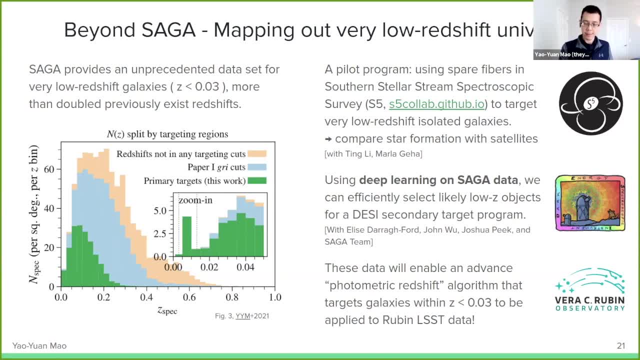 using the Vera Rubin Observatory LST data sets And, in particular, I'm hoping that we can use the data we have collected through SAGAR and DESY and develop something like a photometric ratio algorithm that actually works well in the very low-ration regime. This has been 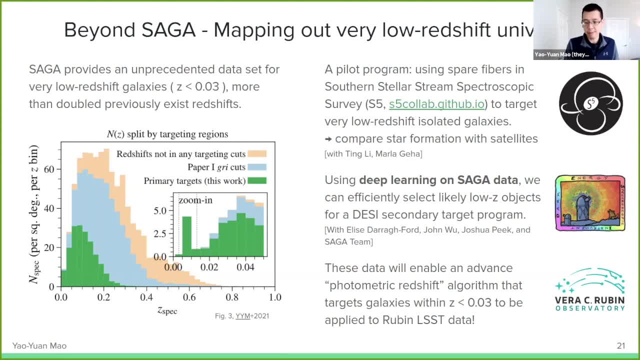 very difficult for a regular photometric ratio, not because of the odds, but because of the algorithm, but because of the lack of training data, And so the hope is that, with all the data we have been getting, we were able to create something like a photometric ratio algorithm. 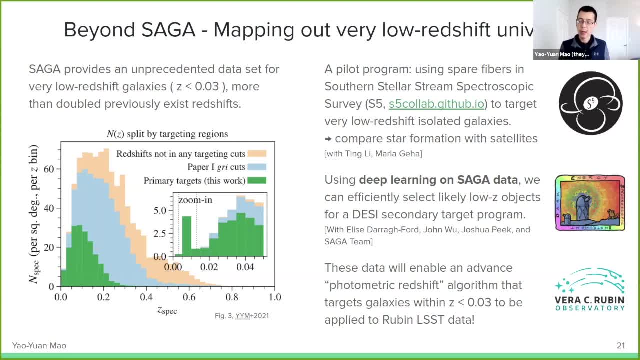 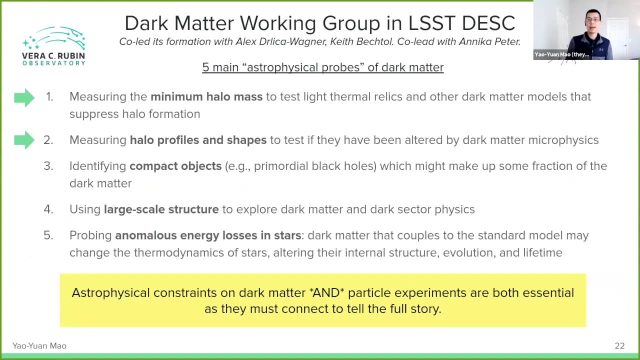 for the very low-ratio universe And that will help us to map out the very low growth galaxy in the universe and map out the structure at that particular mass range within the local universe And that will actually help us to understand dark matter. And so this is: 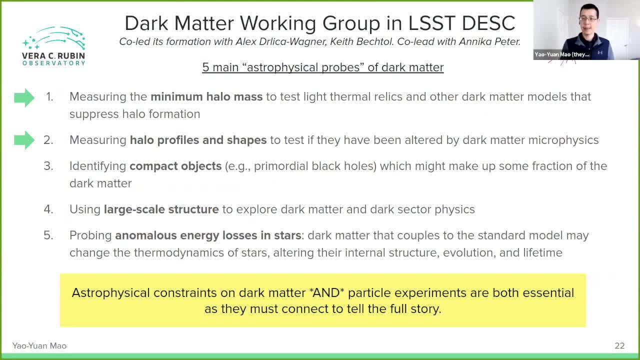 as I mentioned. as Shirley mentioned, I'm leading the documentary working group in the Dark Energy Senses Collaboration, And the reason I want to map out the local universe in this Rubin LST data set is because they will help us to measure the minimum halo mass. 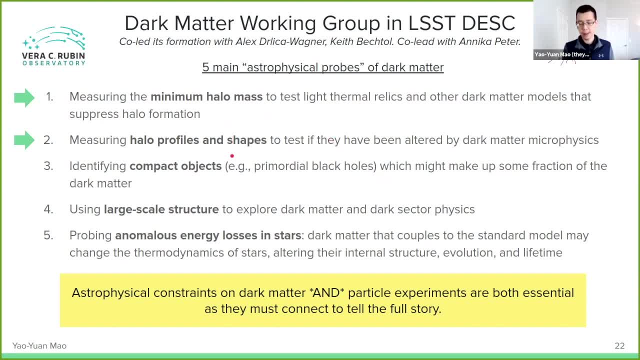 in the local universe And also we can use those very low-ratio dwarf galaxy as lengths and major the weak lensing structure of these dwarf galaxies And they will actually allow us to measure the halo profile and shape that particular sensitive to the self-entered. 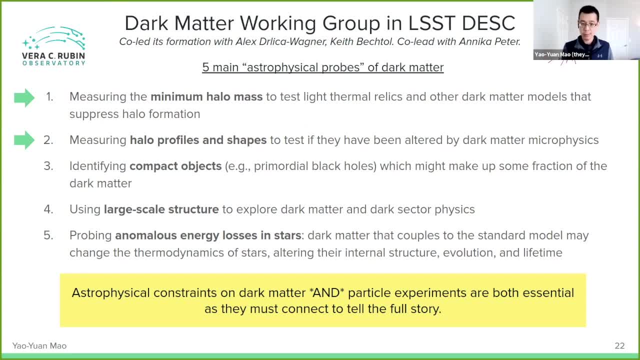 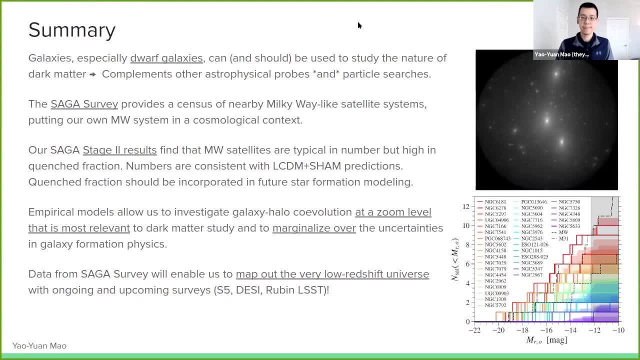 documentary models in these dwarf galaxies. So with that, I'll just put up my summary and take any questions that you might have. Thank you, I'm just going to clap for everybody. Sorry about that Zoom version of clapping. Thank you so much for giving us such an amazing talk. 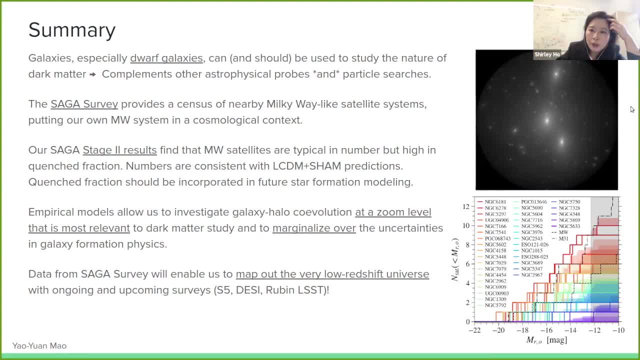 We're going to open up the floor, if you like, for questions. I know people can get very excited. Amiyo, you have a raised hand. You want to go ahead? Yes, I do. Thank you, That was really fascinating And this survey is really 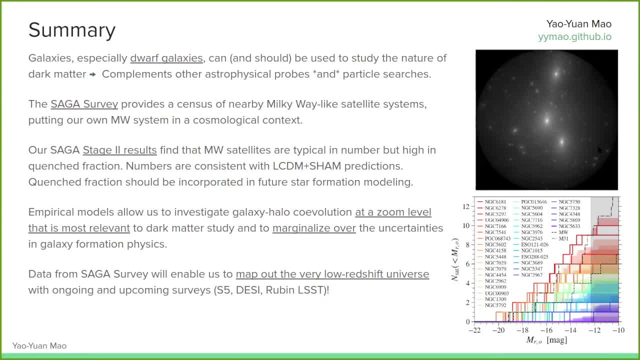 interesting. I have two questions. One is beyond just distinguishing between warm dark matter and cold dark matter. can you use this survey to distinguish between cold dark matter particles? That's my first question. My second question is: can you use the MagSERV survey to? 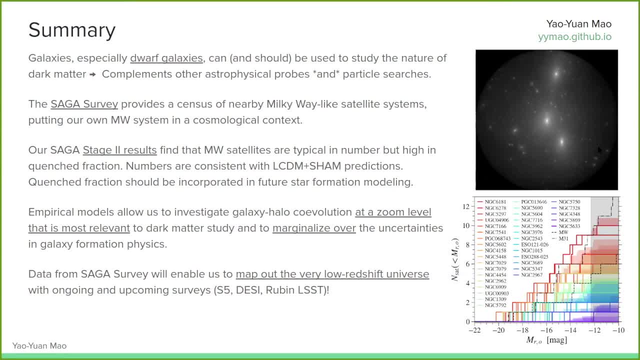 estimate the total varial masses of the parent galaxies around which you see the dwarfs? Yeah, yeah, Thank you. So the first question: between different cold dark matter scenarios, it's difficult to use galaxies to distinguish them Like if they don't actually have an imprint on the underlying structure of the galaxy. 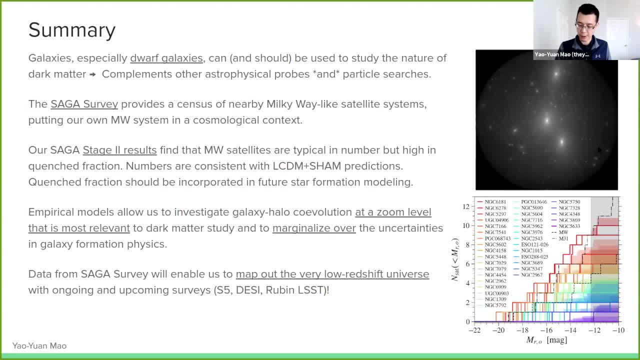 structure of documenter, then it would be difficult. So, for example, if we are talking about WIMPs of different velocity- sorry, different masses- that would be difficult to tell from a galaxy alone. However, I also think that understanding the galaxy-level 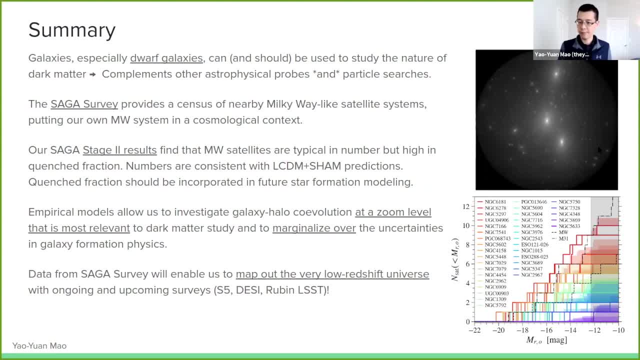 connection better will help us in other experiments, For example, if direct detection is going to measure different co-documenter particles right and that also requires a better understanding of, say, the documenter halo of the MQA itself. And that is where this kind of starting galaxy-level 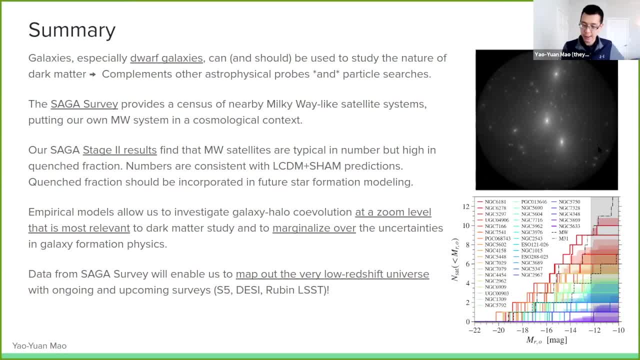 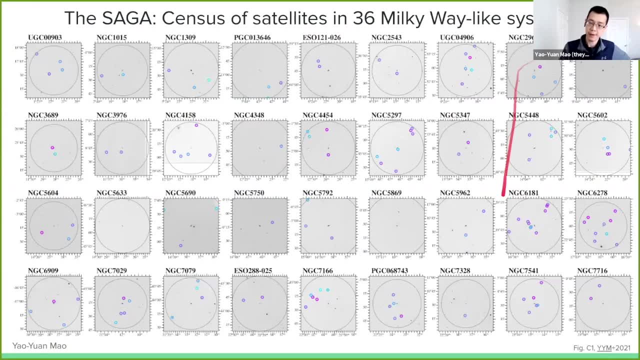 connection will help. And the second question: yes, certainly the satellite can tell us a little bit about also the galaxy-level connection of the host halo. So this plot I'm showing here, for example, this is all the velocity colored by the velocity of the satellite. 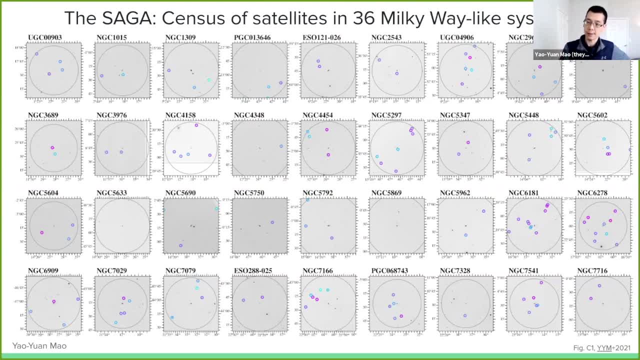 So that will give us some dynamical mass of the host galaxy. so host-documenter halo also. Now, this is only line-of-sight velocity. We don't have the transverse velocity. We are also hoping to obtain dynamical mass of the host galaxy. So this is only line-of-sight. 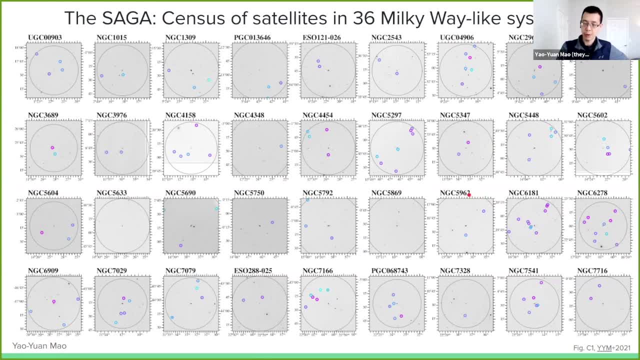 velocity. We don't have the transverse velocity. We are also hoping to obtain dynamical mass from gas of all this individual system. We will want to do a follow-up program for this and actually we can then compare the dynamic mass from gas and dynamic mass from satellites. 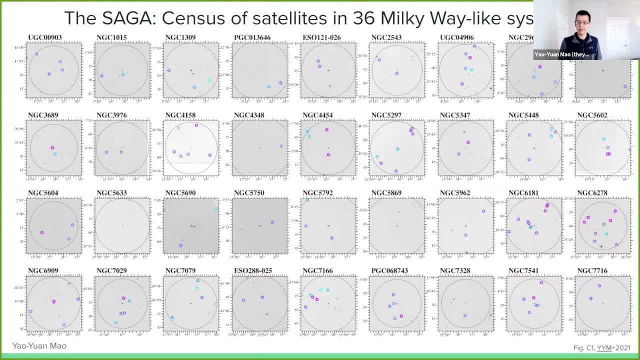 And that will also help us learn a little bit more about the documenter system of the entire system. Thank you so much, And I just wrote down the sequence because there's so many questions, There's so many raised hands, so I just wrote them according to the time they pop. 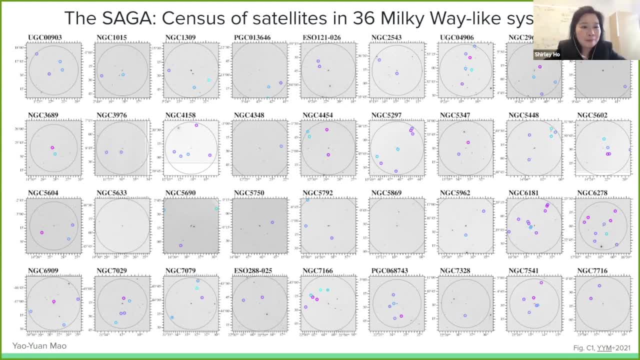 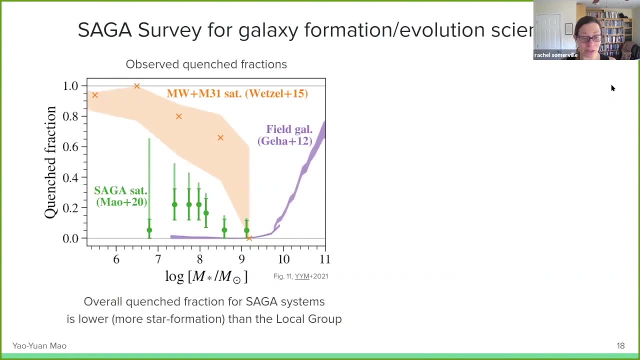 up, at least on my screen. So, Rachel, please Thanks Yao. Great talk, Great stuff. So I'm really intrigued by the fraction of quenched satellites. That's always been one of the most interesting results to come out of Saga And so 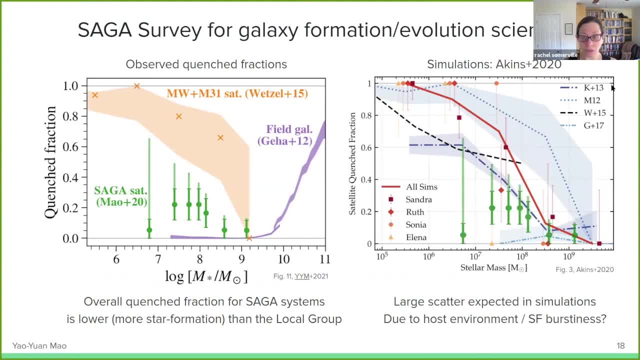 it's interesting to see that persisting. So what I'm wondering is, now that you have this beautiful suite of simulations, where some simulations are showing a high quenched fraction and some are showing a low quenched fraction, can you go in and tell us why you're getting those results? Does 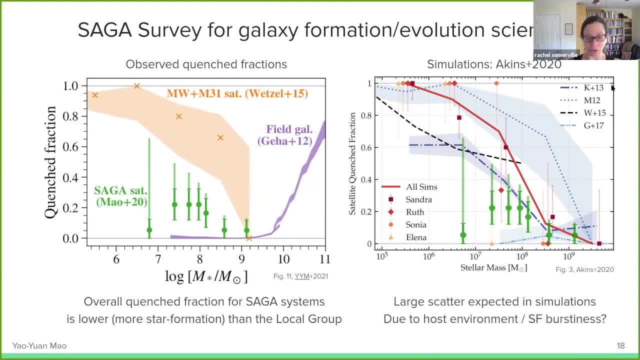 it have to do with the orbits of the satellites? Does it have to do with, you know, something to do with the cosmic web or the orientation of filaments? What is the physical cause of this result in the simulations? Yeah, certainly. Thank you, Rachel, And this is also one of our most. 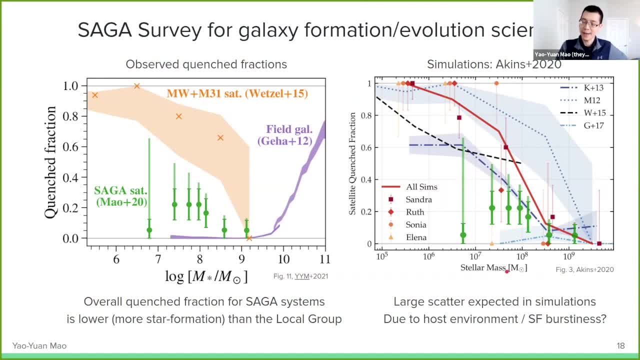 I guess interesting questions, Kind of Saga survey. So, as you can see my note here, I would say my first guess are either the environment and or the persistedness in star formation history, And the reason is that. so first of all we definitely want to do this, but it's still a little bit difficult at this. 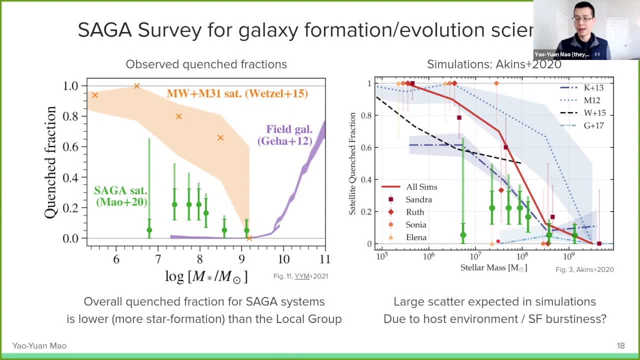 current stage, just because actually the simulation we don't have like a large number of populations. So you can see there are four here. We are actually also excited about the TNG50, which is coming out just recently and want to do a 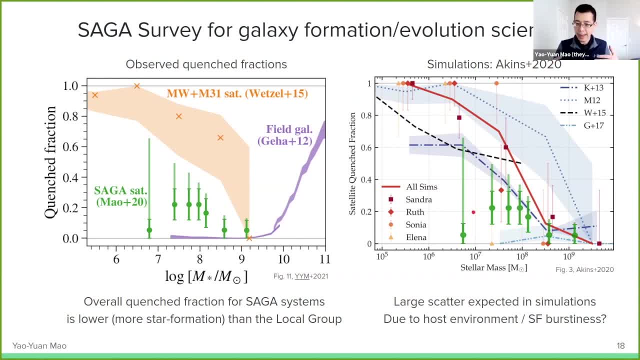 comparison there as well, And but. but I think by the end of we have a hundred system, we will also have a lot more simulation that we can compare Among the objects that we have compared. So I'm working with Alison also about this. Environment definitely seem to have some impact. 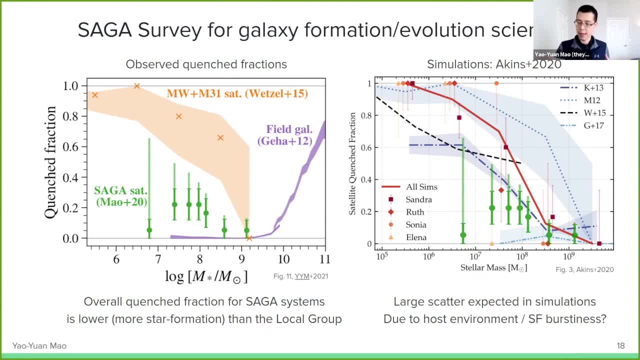 So, for example, if we see you have a companion M31, like companion, or the host itself is older, like a phone. earlier it does seem the satellite are more crunched but this is not yet statistically significant. just because the number of systems we also find the 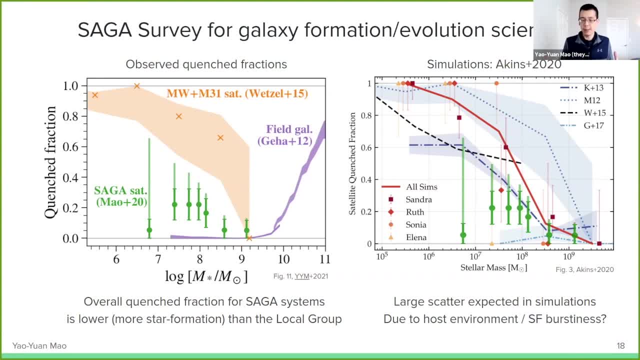 person is quite interesting because in some cases we just don't see any correlation between the system that are more crunching, less crunched, And we were just wondering if that could be just due to the person. It's like we happen to see a snapshot of things, that they are crunched, And so 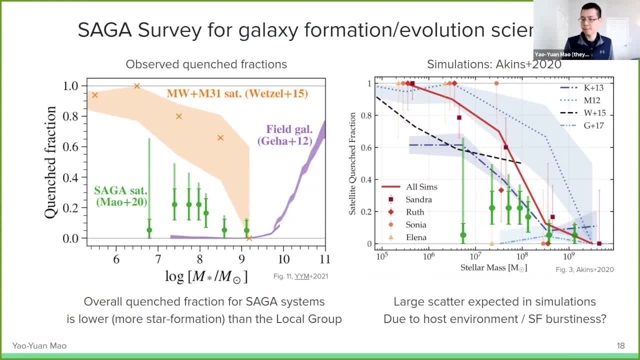 for that we can also actually just estimate it. So in order to see the chart, you can look within the fragment of you know more crunched assistance and compare it with you know quenching timescale and see if there's difference can be explained. 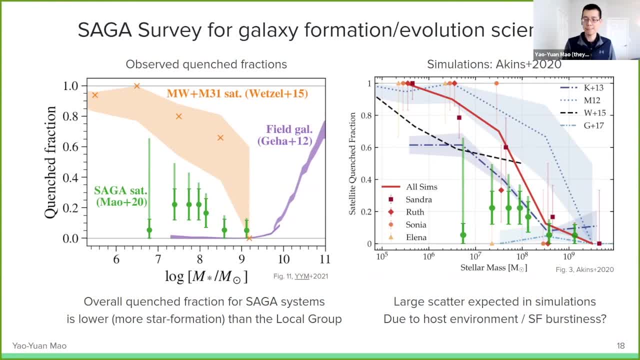 So this is one of our top priorities in the upcoming study. Great Thanks, Joao, That's fascinating. Thank you, I think next up is Alberto. Thank you, Joao, for the talk. So just a very basic question, Do you see? 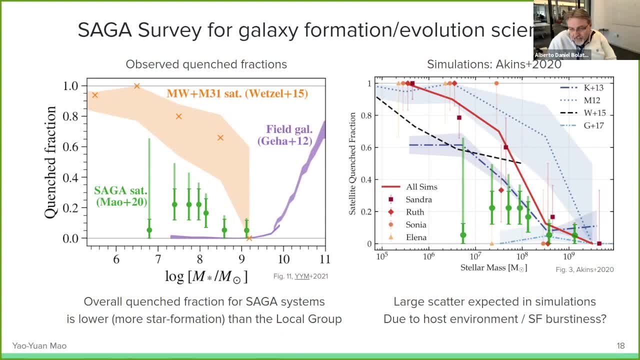 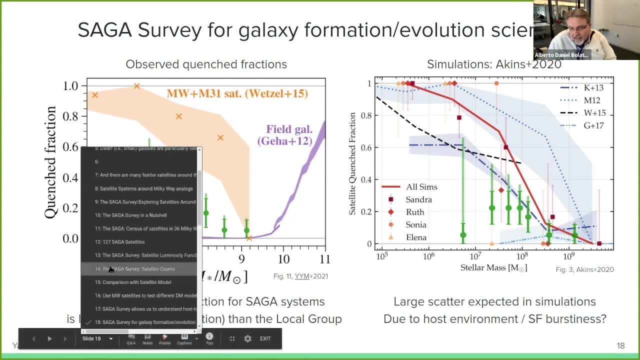 I hope you analyze the data for the presence of favored planes and the even that you have the kinematics and the distribution of the satellites, And do you see a relation between that and the spin of the central object, et cetera? Great question. 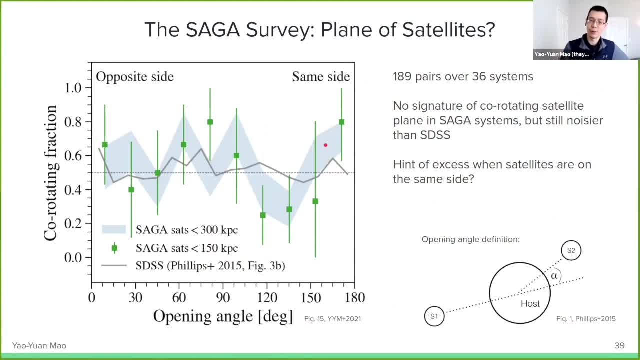 We don't quite, yeah, So okay. so just let me recap for people who may not- if you're not familiar with there has been this very, I guess, heated discussion about whether there's a planar structure, like in the MQA, M31 and many others that are systems. 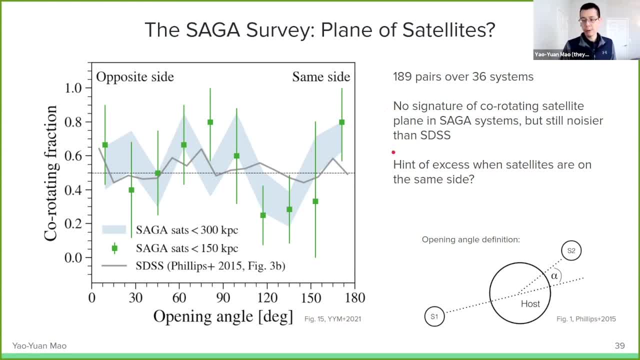 So in the Saga survey we did, like another study, which we look at the satellite pairs and then we plot whether they are moving in the same direction or the opposite directions, as a function of the opening angle. So this means those two satellites are on the opposite side of the host. 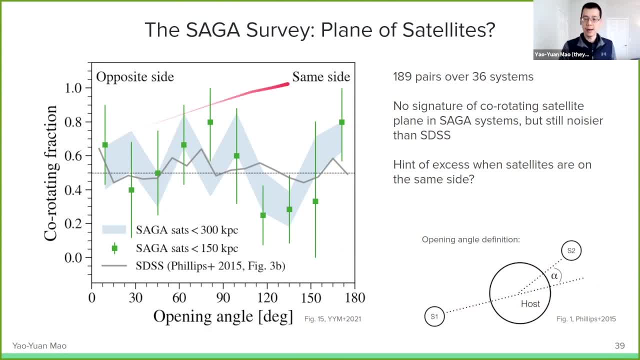 and they are moving in the opposite direction, So they are co-rotating the other way. So this means the two satellites are on the same side and they are moving to the same direction, And so you can see the Saga points in green and blue bands. 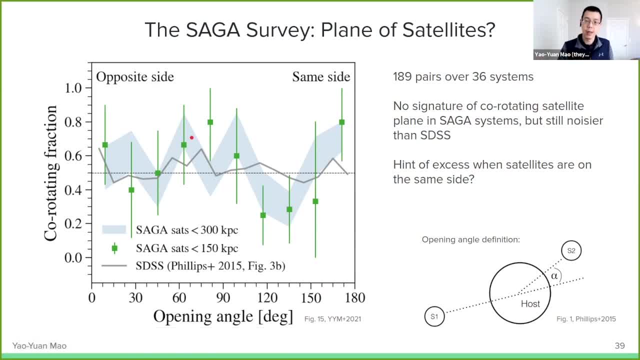 they are just satellite. they are in the inner region or outer region. We don't really quite see a very strong signal. as you can see, There seem to be some. I wouldn't, I don't know. actually, this is the plan of satellite. 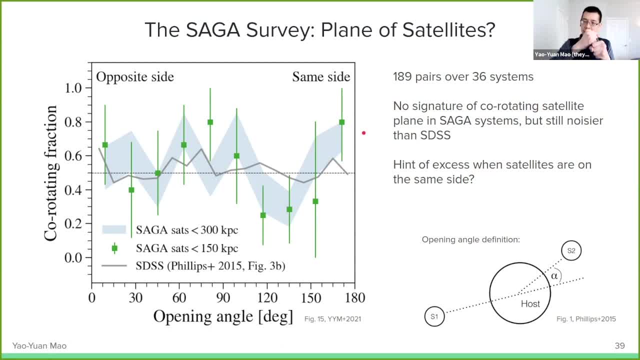 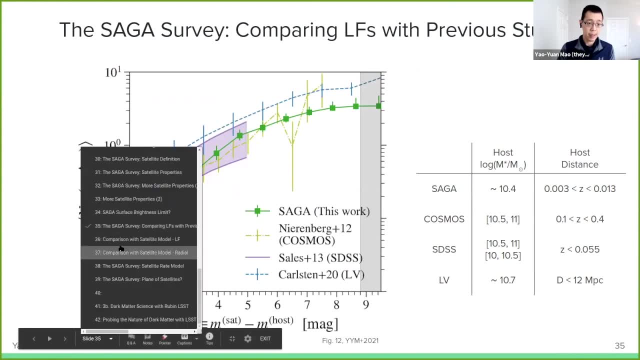 or more like co-rotating pairs. We still see a few satellite that are really close by and they're moving to a same direction, So I can actually let me just jump back to this. Like you can even see some of this here, right? 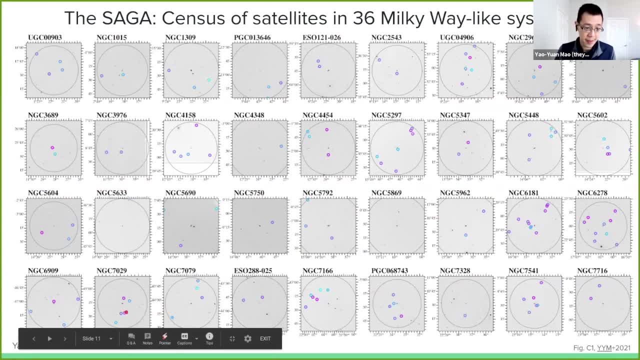 So, like you can see, like this pair, they have a similar velocity and also very close to each other. You see some of the pairs here. they are very close to each other and have very similar velocity And just you can draw by eye. 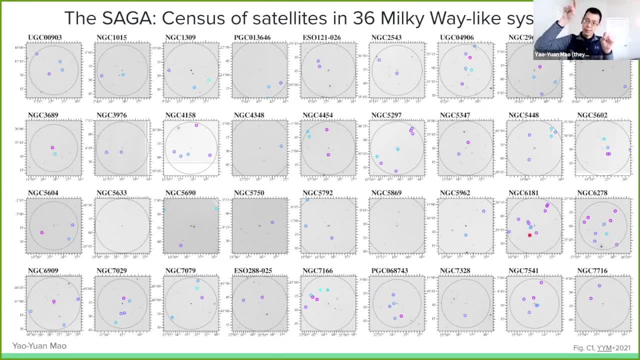 like a few like this kind of pair, And that is what like drive the bump that you see earlier. But otherwise we don't see a statistical significance of a plan of satellite for now. If you run the same test on the simulation so you get anything different. 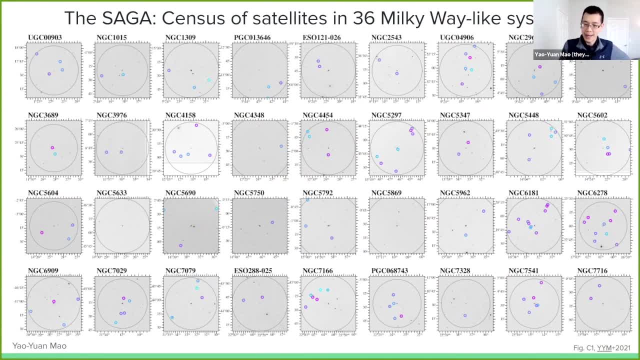 So that is part that is a heated debate, I guess. So my own study of a simulation that I ran: we don't see a signal of plan of satellite, but there has been debates about like whether, how you do statistics and whether, like 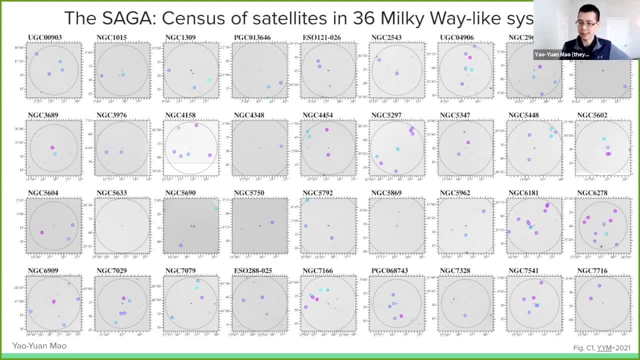 if you plot the statistic in a certain way, you will see a signal or not see a signal, But so far I haven't been able to find a strong signal in simulation that I have run. Okay, thank you. Thank you so much. 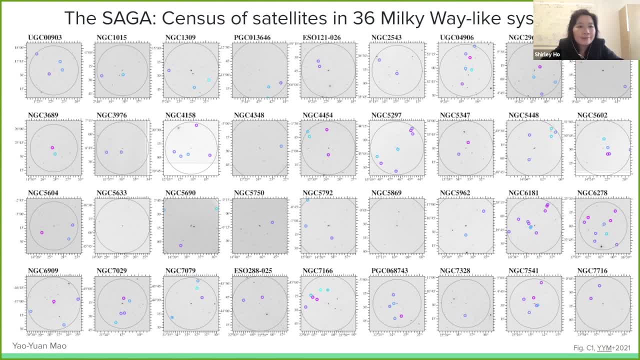 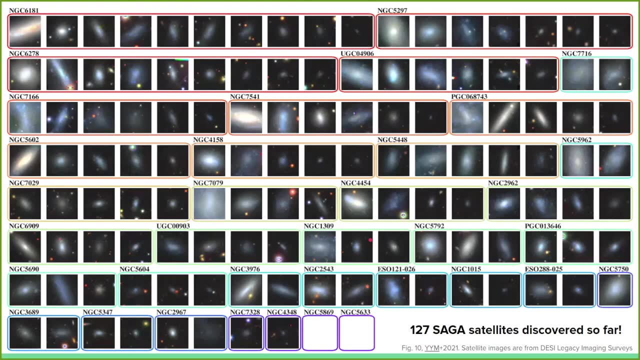 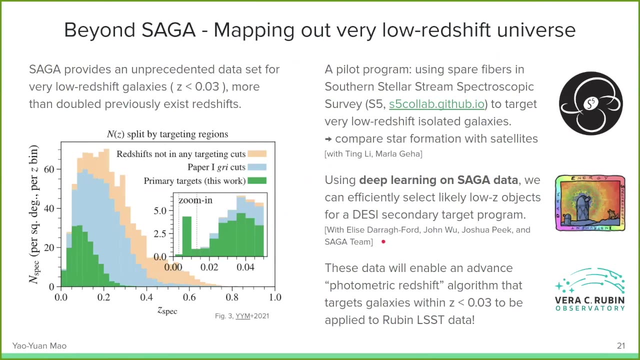 So who's up next? Leman Hi, thanks for the talk. You mentioned the DESE secondary target program, which seems great for this application, And I was also wondering in the within DESE if the bright galaxy survey would let you do some of this as well. 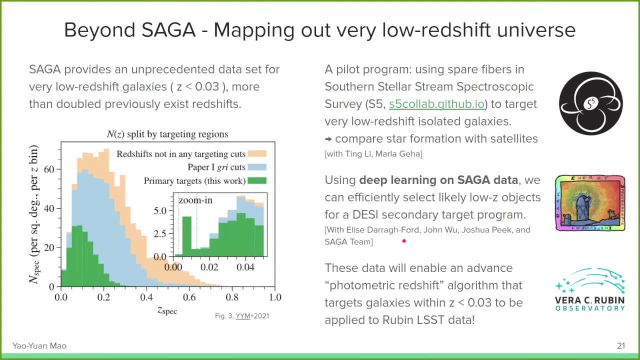 maybe extend it to a little bit higher redshift? Yeah, certainly. So we are obviously working closely also with other people in the bright galaxy survey. And so just for context for other people, if you're not familiar, the bright galaxy survey roughly go down to: 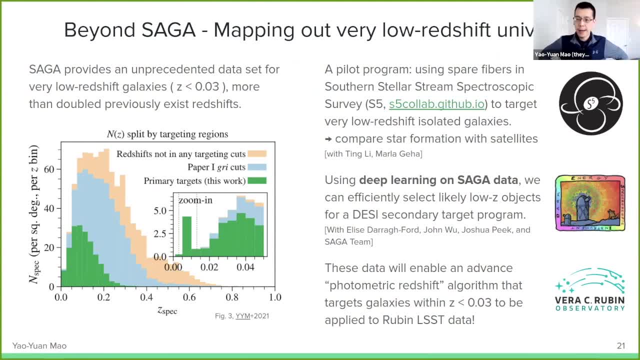 of 19 to 19.5.. And the secondary target we put in roughly cover from the range of 19 to 21st, And so the fact that there's a small overlap is indeed to just compare notes between the bright galaxy survey and our survey. 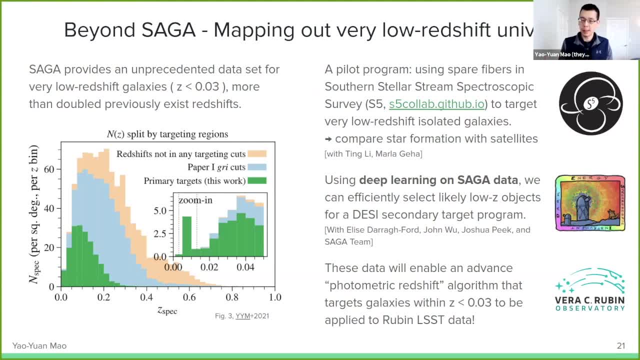 The bright galaxy survey. it's trying to be more complete in terms of everything to the magnitude, And the particular lowly survey we are doing is only going to survey the lower universe, So we are not doing high ratio stuff. But the other thing to note is that 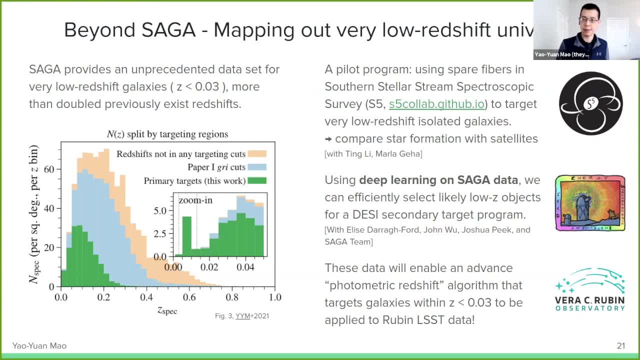 bright galaxy survey is done in bright time And so the secondary survey we are doing is at dark time, So that because it's, But definitely the hope is to join all the information we have available, including the bright galaxy survey and the lowly secondary target. 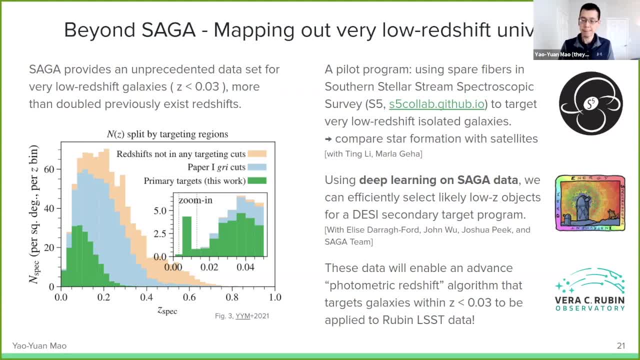 And so that's what we're trying to do with this program: to understand the evolution of the galaxy. Great, Thank you. Thank you. I feel like I want to jump in with a quick question, But, Josh, you can go first if you like. 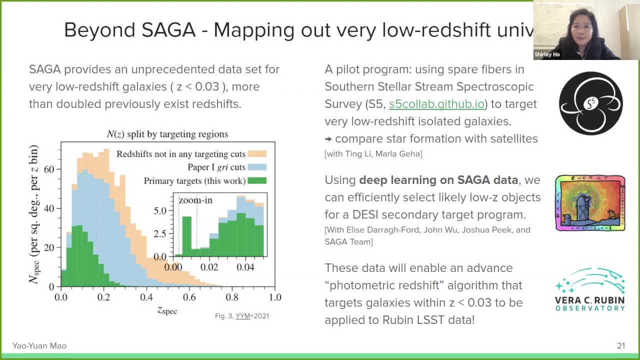 I'm the host. I can go last. Sure, Thanks, Shirley. Yeah, Thanks, You have a great talk, So I just have a quick question about like these. So have you ever considered looking at the halos that are lower than like 10 to the sixth solar mass? 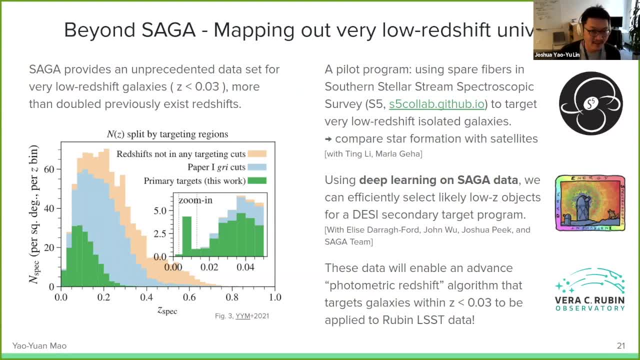 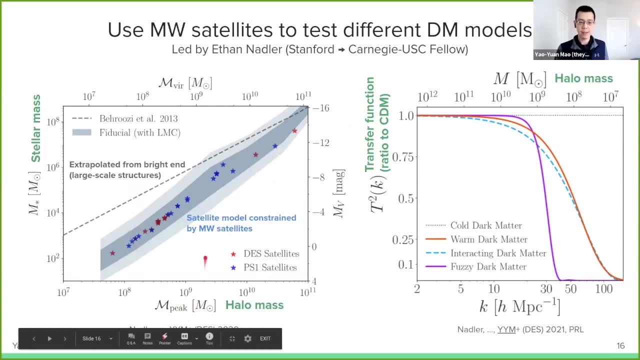 Because I think there's going to be lots of thesis problems And would it be interesting to also study in this survey? Yeah, So I mean obviously in the Milky Way, we will extend this with, for example, LST data. 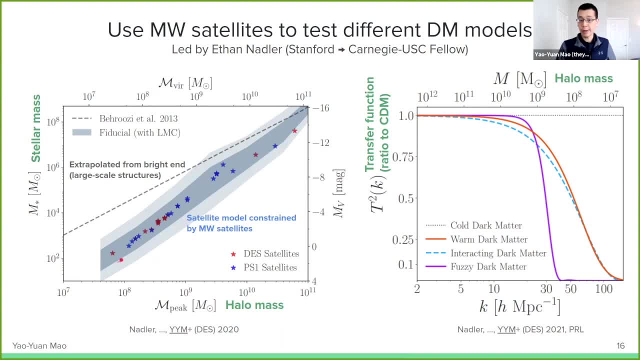 We'll definitely extend this within the Milky Way Also. the Milky Way is going to be really difficult, right? So the program: right now we are trying to calibrate the Milky Way using the bright end, just because the satellite function is a very nice self-similar. 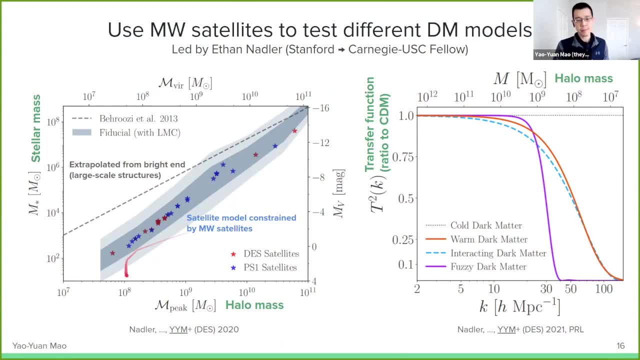 function So you can calibrate the amplitude using the bright end. But if we want to go to like 10 to the 7 in stellar mass- sorry, in halo mass- that means you are talking about 10 to 100 solar mass in stellar mass. 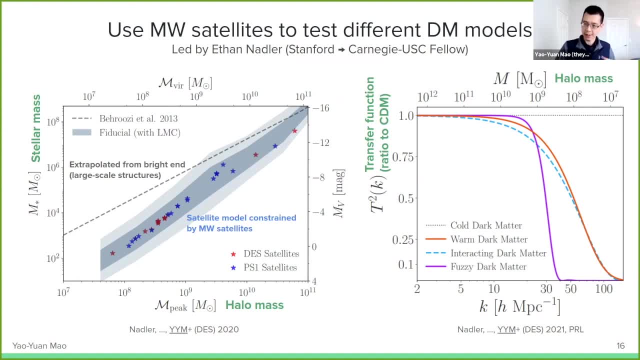 That is still prohibitive right now for things outside of a local group. But yeah, we are thinking of this. We have been talking with people doing follow-up observation using HST in specific solar field. We are talking about using PFS on doing again. 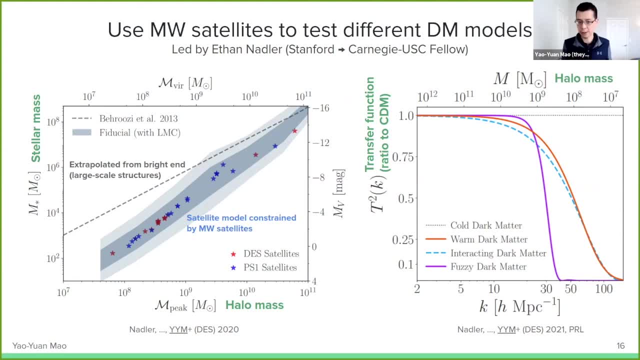 a target observation for one specific field, But it's difficult to do it for more survey, for more system at that magnitude limit. Thank you, Anyone else want to ask a quick question Or I can start with my first. All right, Yao, you simulated like 45 galaxies, to compare. 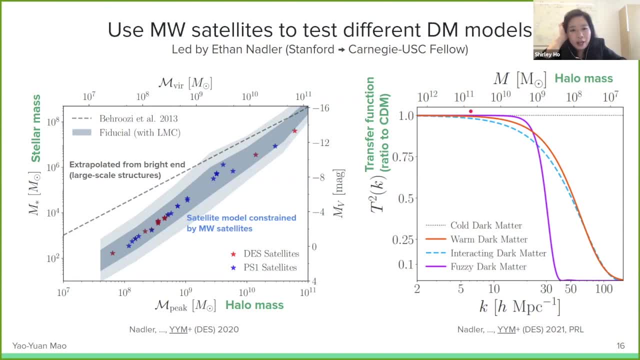 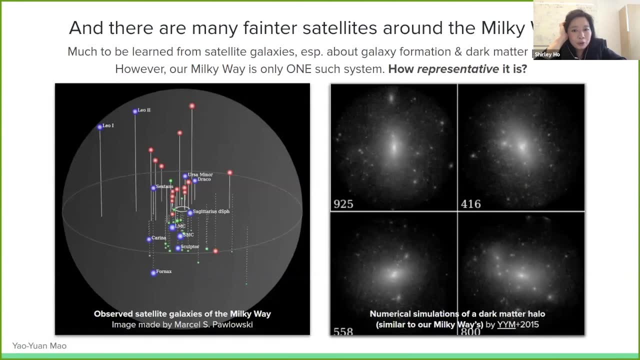 to a Milky Way at the beginning, And then the question I had in mind immediately was: how do we know for sure we have simulated enough sort of diversity of galaxies compared to a Milky Way, And what would be your dream number of galaxies you feel like you need to generate? 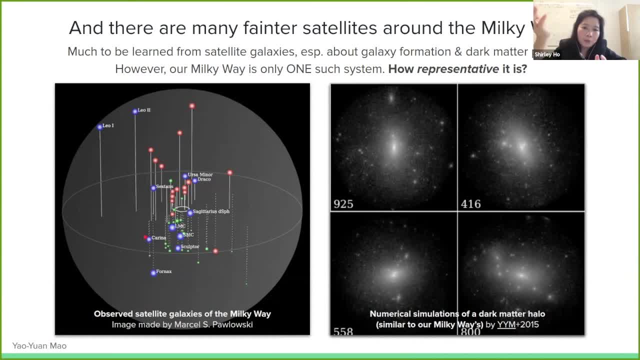 And that relates to another question, which is for this program to work to understand the properties of dark matter. we kind of need to understand the degeneracy possibly between the galaxy formation history and environment with the properties of dark matter, and what are your plans on that direction. 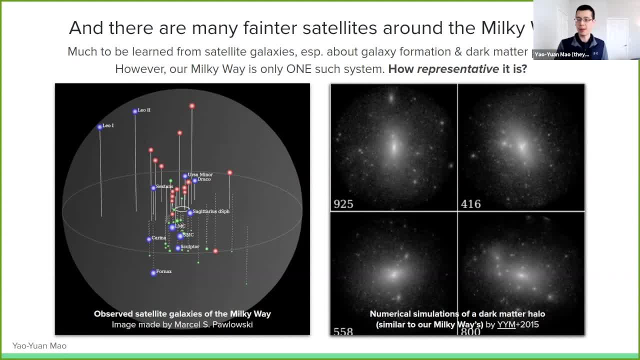 Yeah, Great, Thank you. So the first question is on the number. 45 is not too bad, I can say. we started to want to do 100. And in the end we found that actually what is more important is to characterize how the amplitude correlate. 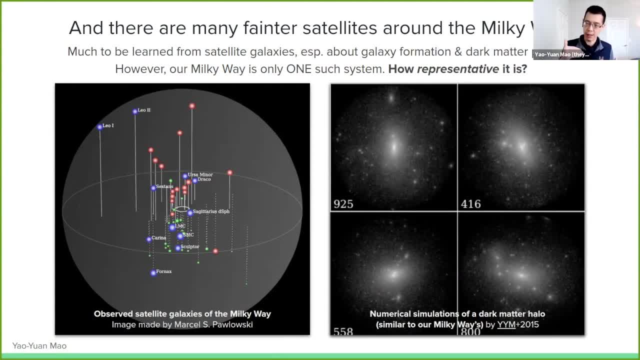 with a specific property of dark matter halos, For example, how the satellite amplitude correlated with formation time, correlated with the shape or the density of the dark matter halos. Once you characterize this, because in code I made a case, they are really self-similar. 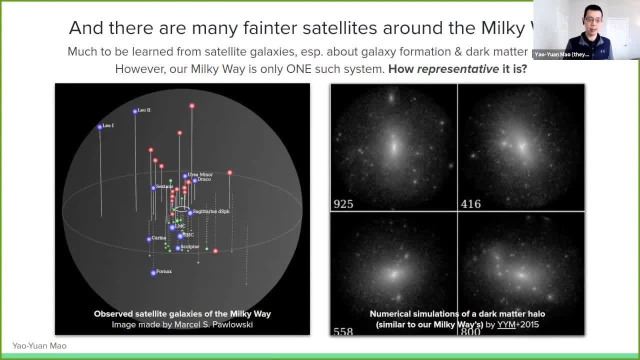 They don't actually. I mean, adding more systems doesn't really add a lot more, I guess. information on that particular part. However, let's say we are running a suite of simulation that are more specific than Milky Way, Like we want to understand a few other things. 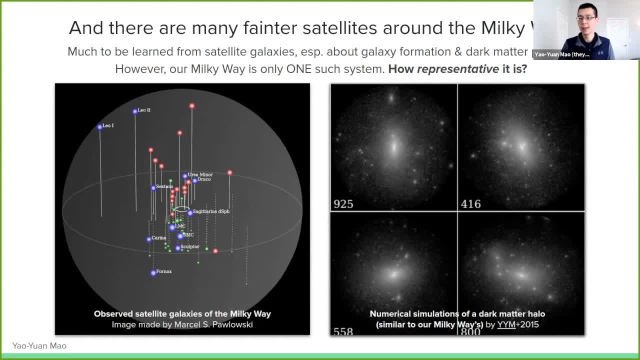 that Milky Way might be different. For example, the existence of LMC. We have found that the existence of LMC seem to be playing an important role in terms of the total satellite population. We also see that I mean the data set as well. 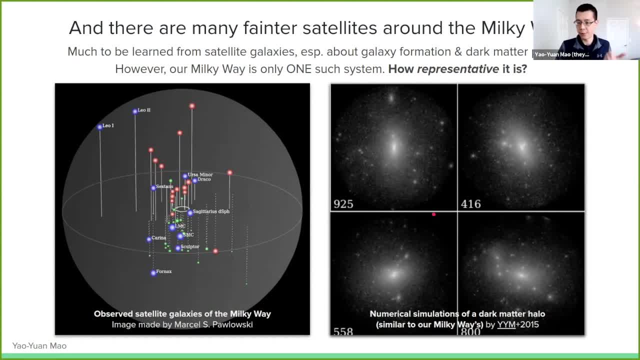 And so we are running a set of simulations which have a recent created bright satellite And hopefully that will also add to this suite and span a wider range of Milky Way-ish galaxies and halos. The second question is: how do we break the degeneracy? 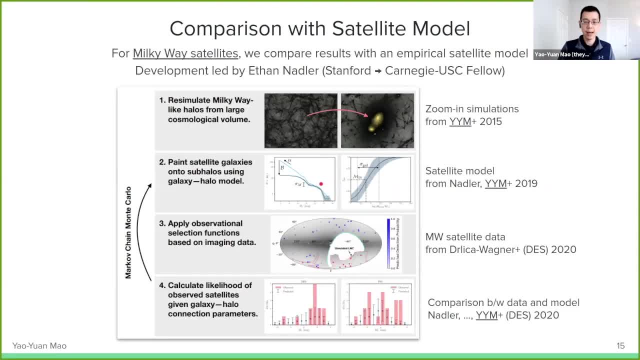 between, I guess, galaxy formation and dark matter models. This is one of the biggest challenges in this program, And so our hope is that this kind of satellite model that I talk about, they act as like a layer that you can marginalize over. 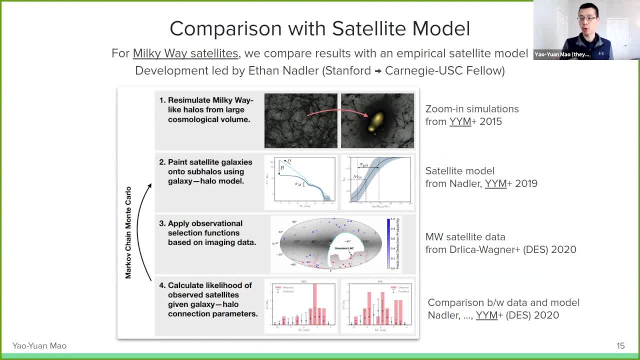 And their prior can come from independent observation and or hydrodynamical simulations. So you can think of hydrodynamical simulation being realizations of specific physical models And you can, if so, depending on your belief, say if you trust certain hydrosimulation. 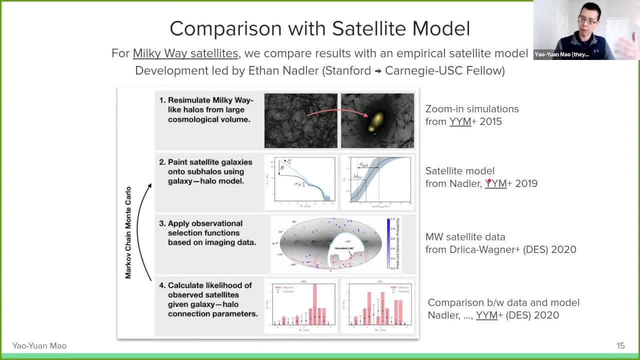 those then give you very strong priors on this satellite model in your program And then so you've got a much better limit in your document, similarly In your dark matter constraint. Or we can say: well, I don't fully trust the hydrodynamic simulation. 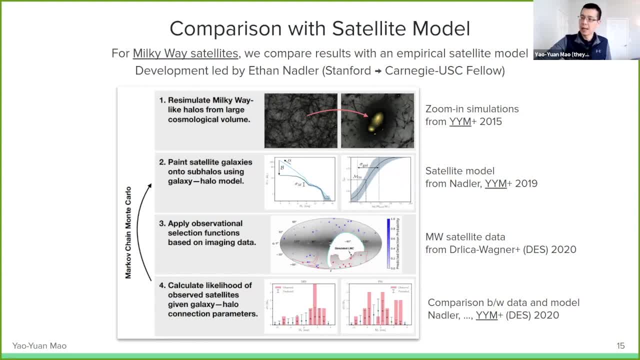 But I got, I don't know, five different hydrodynamic simulation with slightly different star formation prescription And I will take all of this as a prior. They will obviously weaken the dark matter constraint But you have a higher confidence of you marginalize over a broader range of galaxy formation. 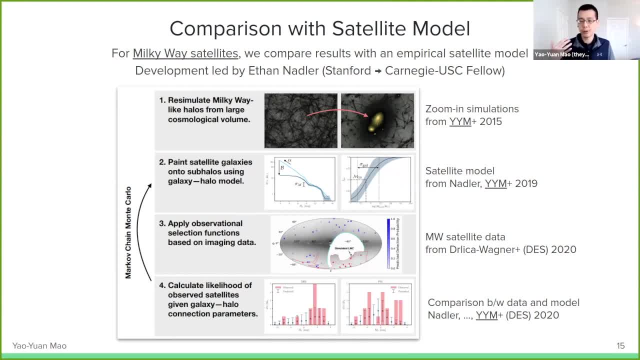 So this is the program I'm having in mind, And so we are hoping to both using independent observation on galaxy formation itself, both from the Milky Way, outside of the Milky Way, and also from hydrodynamic simulation to construct priors for these empirical models.